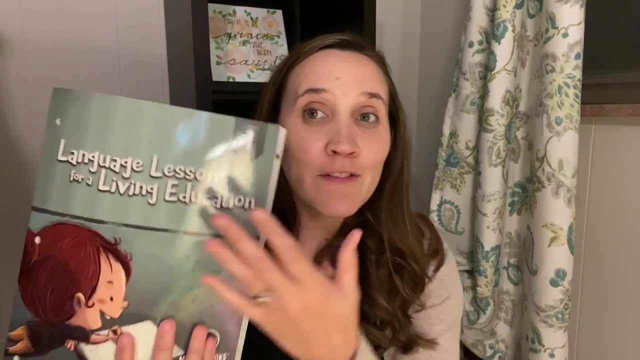 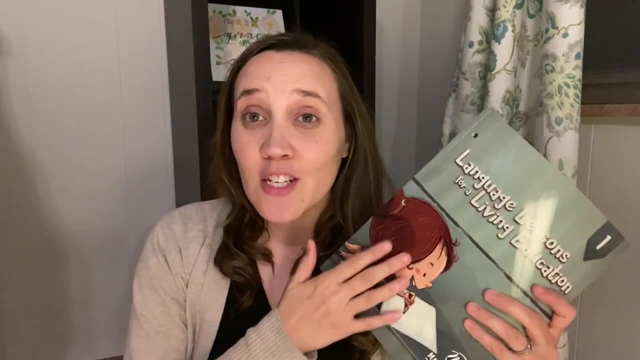 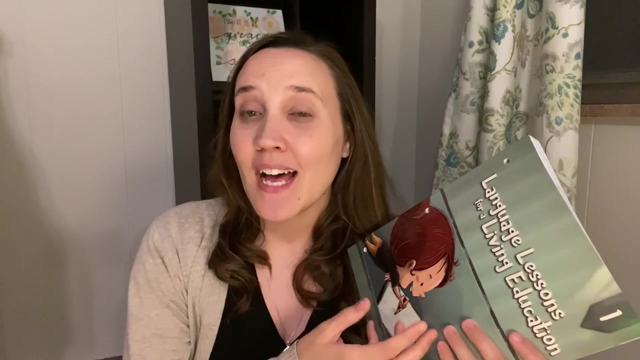 video today as well. that is kind of well. it is themed around this same curriculum. However, what she's doing is she is showing this curriculum in action, So I'm going to show a very in-depth flip through And look inside, and she is actually going to give her thoughts on this and actually putting it into. 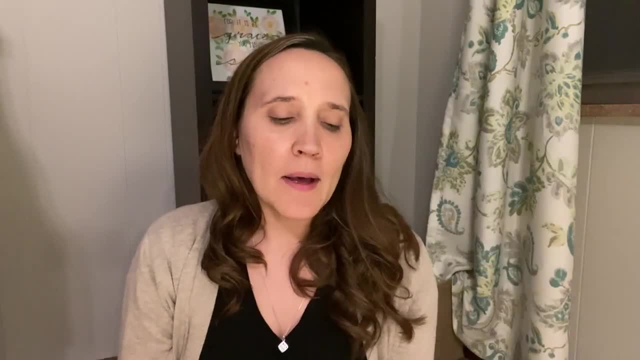 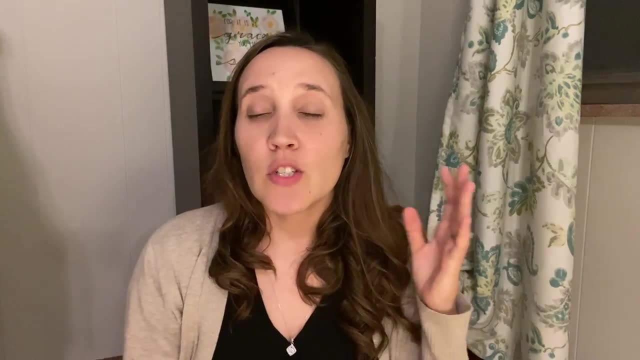 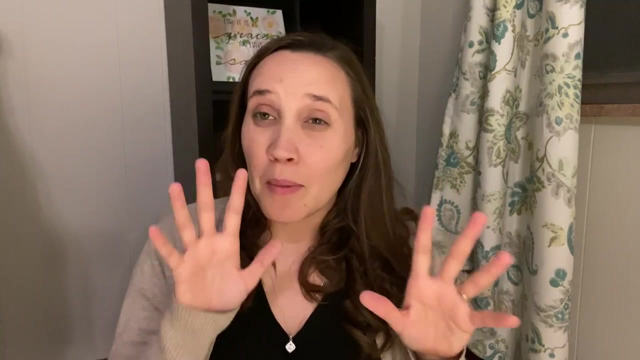 action because we haven't started using this yet And also this also replaced basic language skills that they used to have before, So she has used that as well. So Colleen is going to be sharing kind of like a comparison between the two. So you definitely want to make sure that you check. 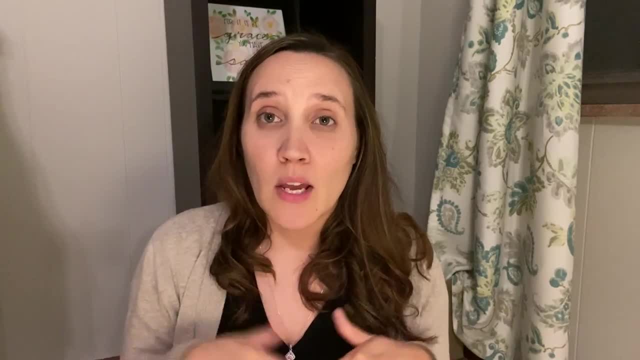 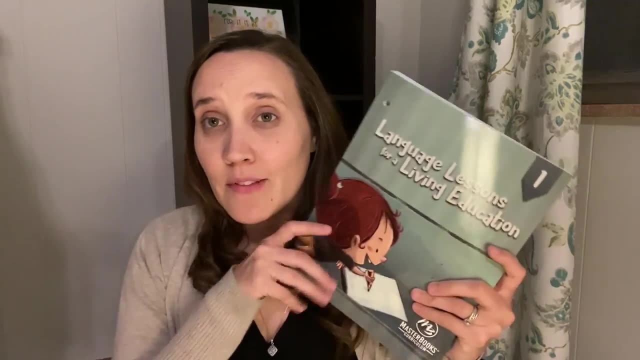 her channel out as well. So I'm going to show you a video today. So I'm going to show you a link to that video down in my description. below I'm going to show you the other books that correlate with it. So you have this, which is the main instruction and worksheets and everything. 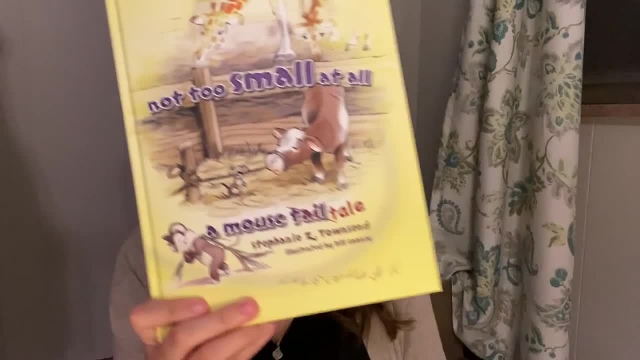 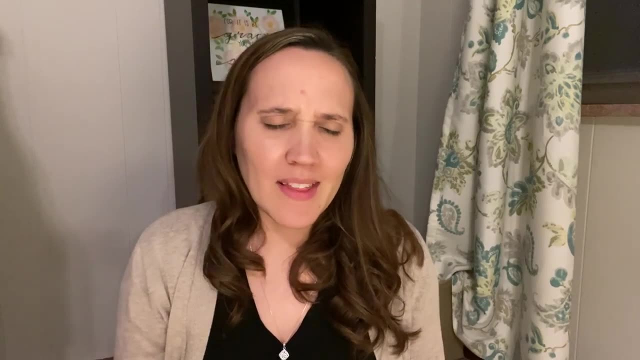 And then you will also use this, which these next three books were actually part of the set- with basic language skills as well. I think I'm saying that name right, the one that this one replaced, So I'm going to show you a video today. So I'm going to show you a video. 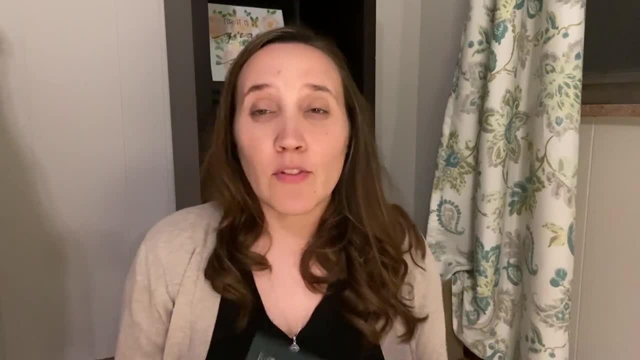 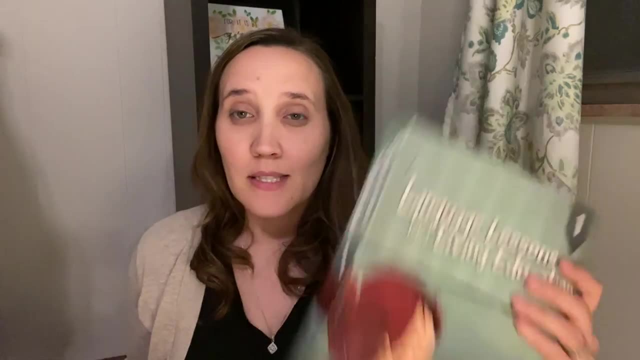 today. So if you have used that in the past, then you of course don't have to buy these next three books. You would only have to buy this. But if you are new to this, you will want to buy these. 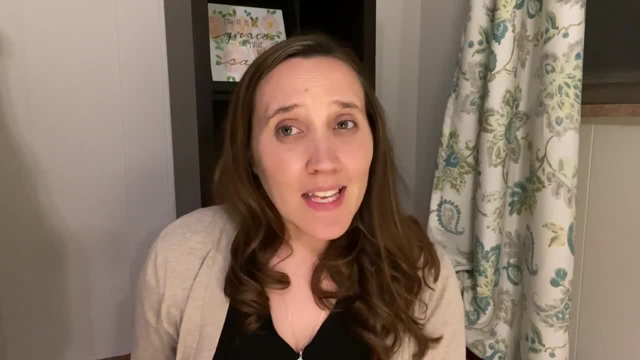 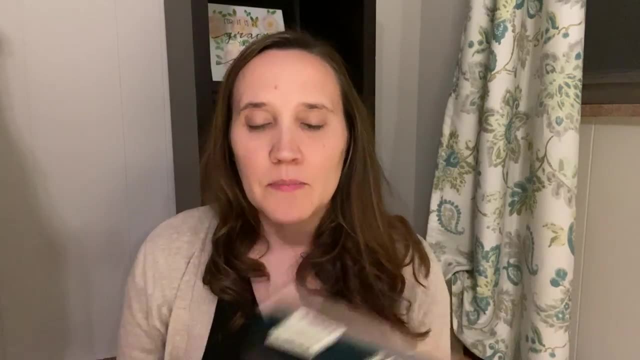 three books because they are used in this curriculum, And I think- only I think- I paid less than like $65 total for all of this. So anyway, so here is oh wrong side. Here is the other one, And I'll kind of show you a video today. So I'm going to show you a video today, So I'm going to 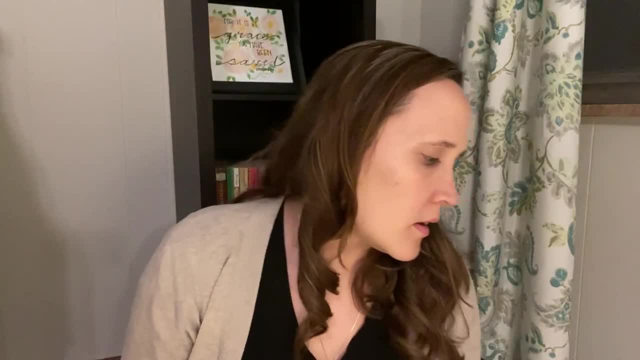 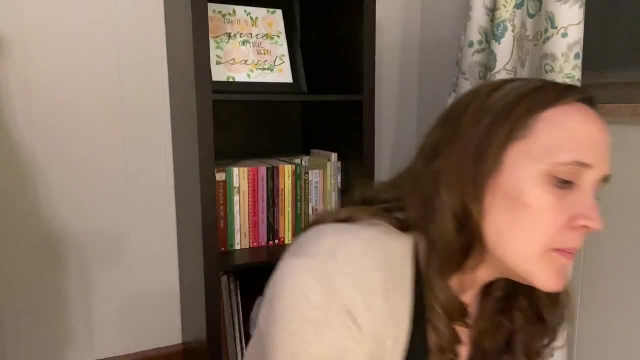 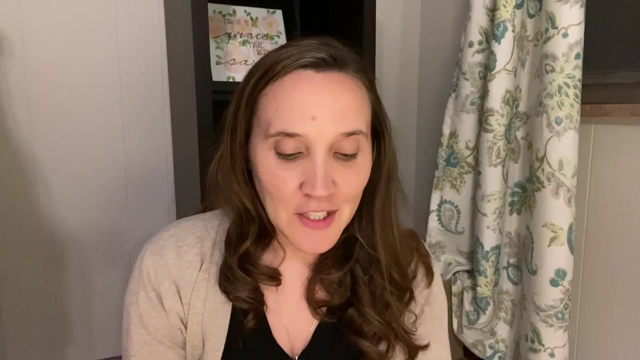 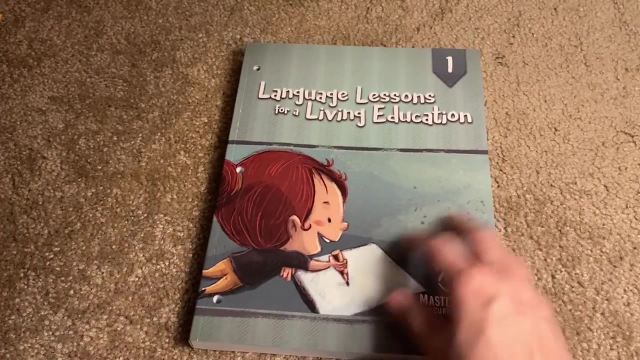 show you looks inside of each one of these as well, And then also this one. So I'm going to turn the camera around and I'm going to show you a look inside of Language Lessons for Living Education- Level 1.. Okay, So here we have our flip through. Okay, So if you are familiar, 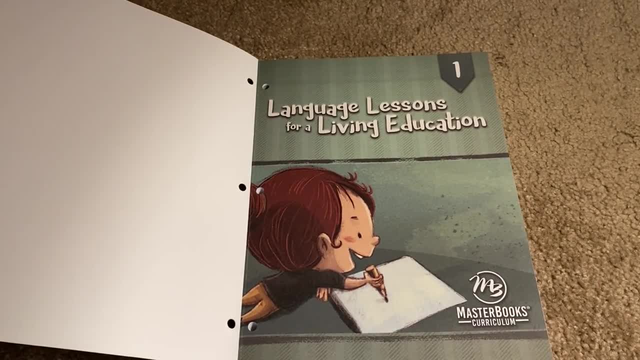 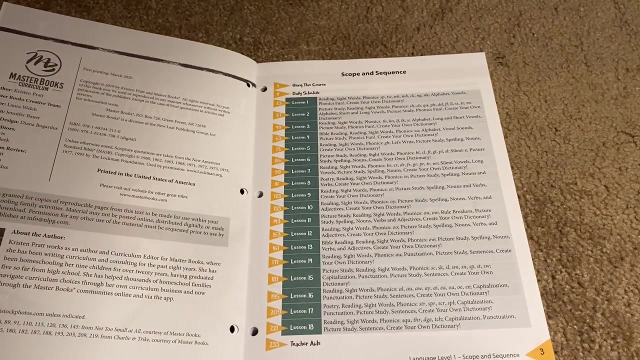 with Masterbooks it looks like. it looks very similar to the inside of my Foundations- Phonics, and also how our we started using Math Lessons for Living Education with my younger ones as well, And so the layout is kind of similar. So the scope and sequence we have here, 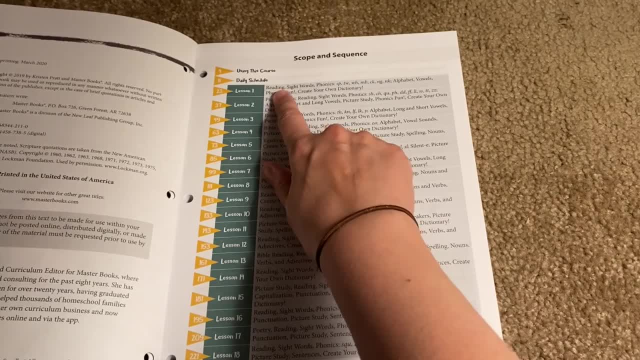 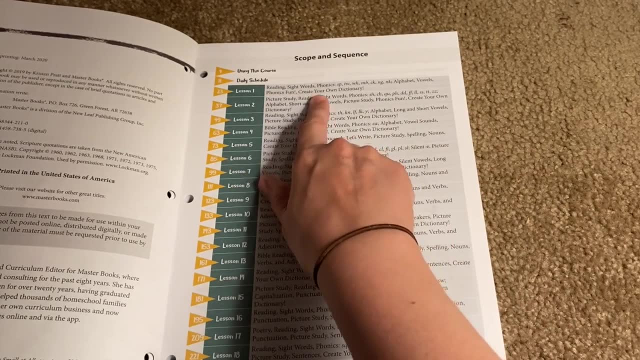 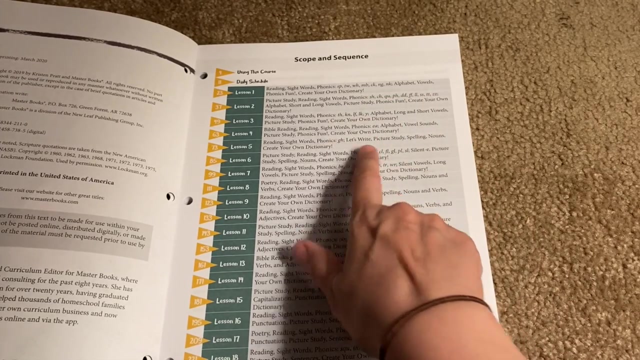 we are going to be. it focuses on reading, sight words, phonics, and it has all your different blends down: alphabet, vowels, phonics, fun- create your own dictionary So they will be working on that. And then so it breaks it down by the phonics blends and sounds that they'll be working on. 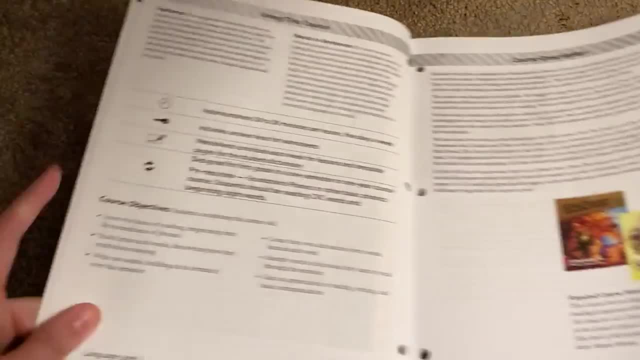 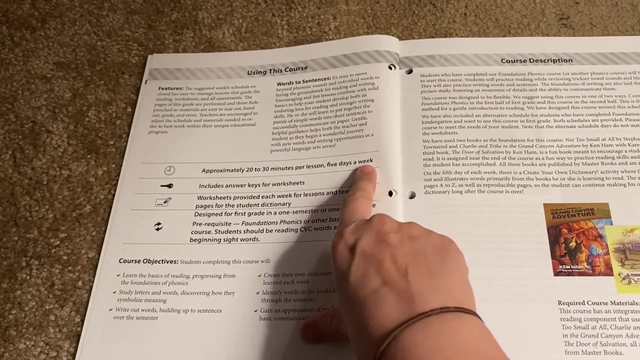 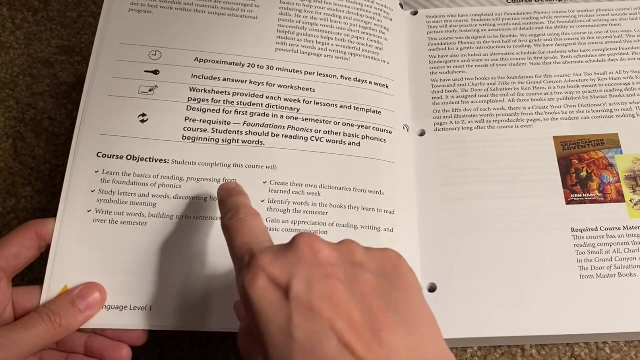 with each lesson, So it has the key. So it takes 20 to 30 minutes per lesson, five days a week. So here are your course objectives: Learn the basics of reading, progressing from the Foundations. phonics, study letters and words, discovering how they symbolize meaning. 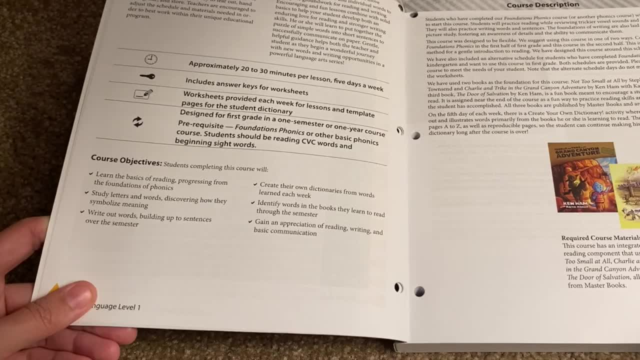 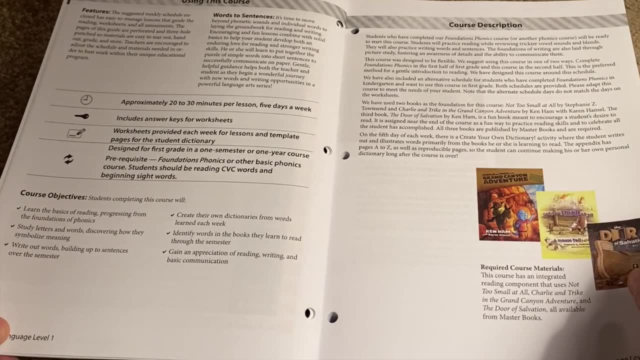 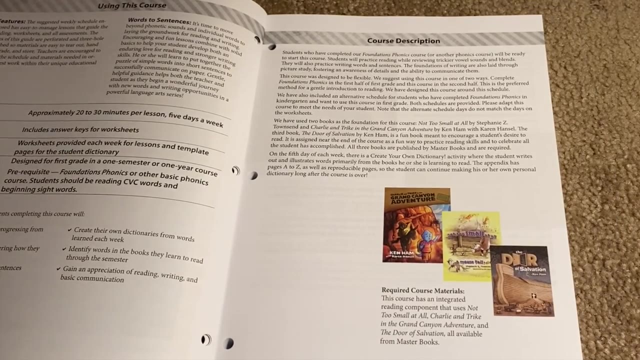 write out words building up to sentences over the semester, create their own dictionaries from words learned each week, identify words in the books that they learned to read through the semester and gain an appreciation of reading, writing and basic communication. So this is assuming that your child has done Foundations- phonics- 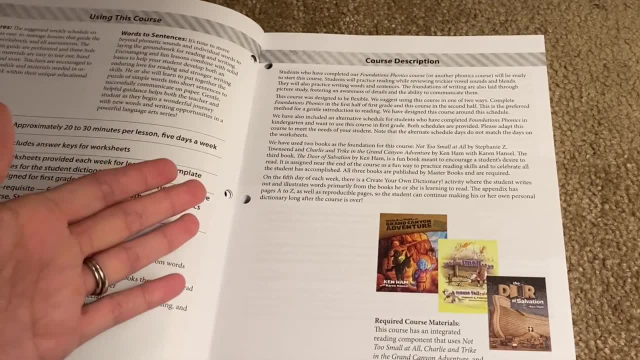 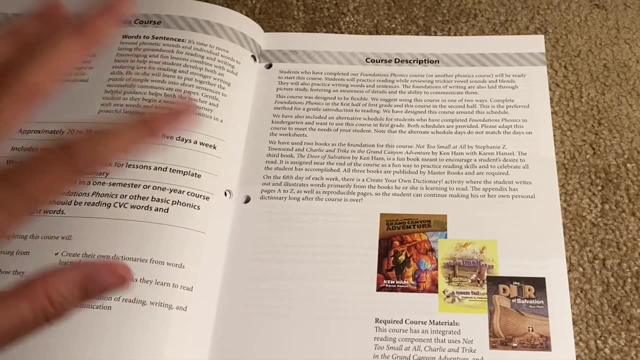 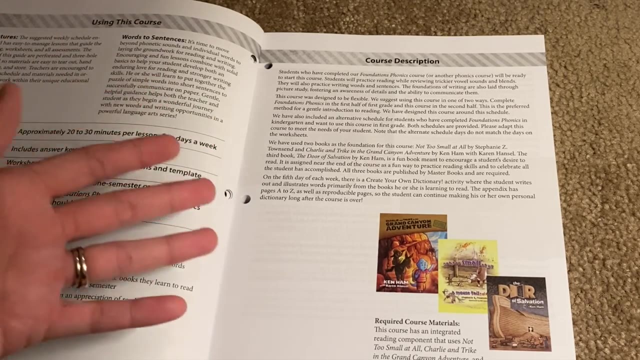 phonics. um. so they want you to start with that um and for the first half of first grade, and then use this for the second half. now my kids that are using this are actually in kindergarten. um, we, like i said, we're currently using foundations phonics, but we're halfway through. 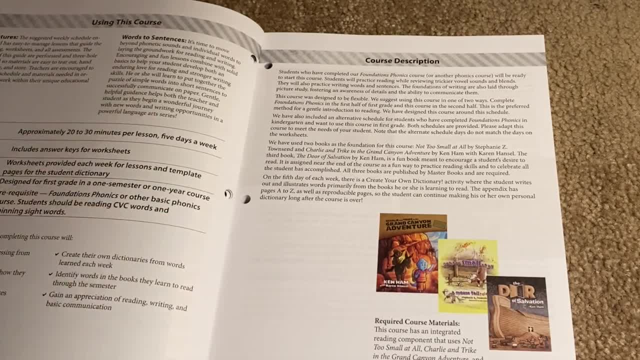 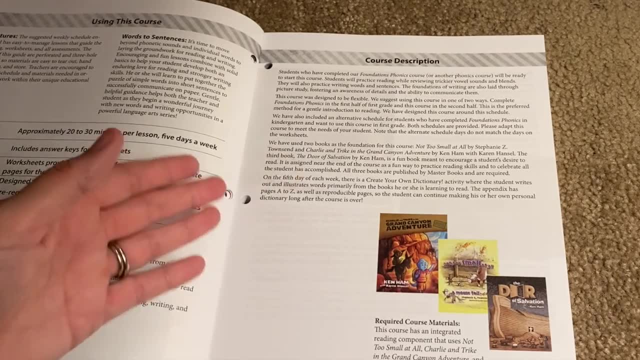 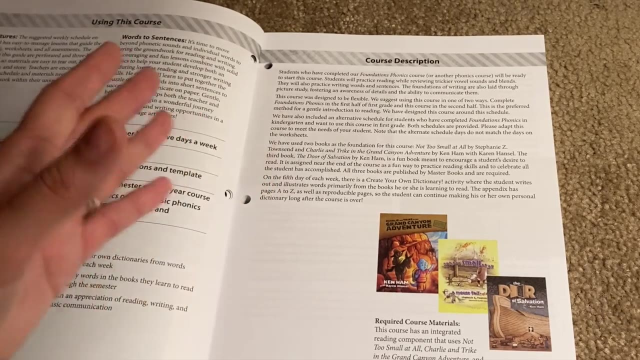 with it and when we finish it we will just go straight into this. so we actually um homeschool year round, so we probably will start this about the time that our official first grade year would start with them, which is in july. but i went ahead and bought it because i was excited, so 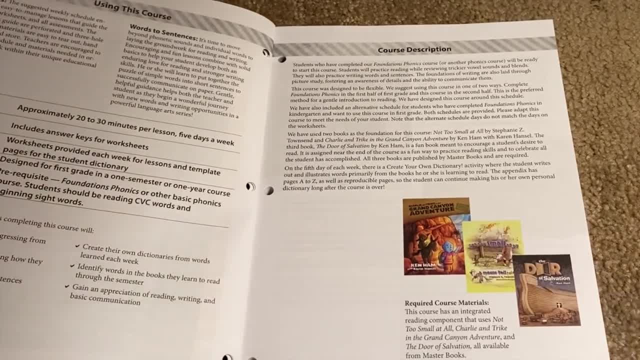 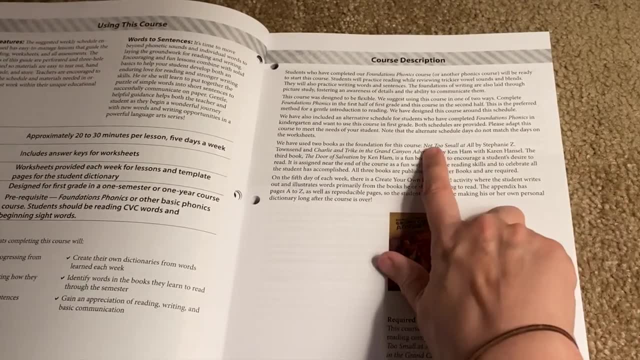 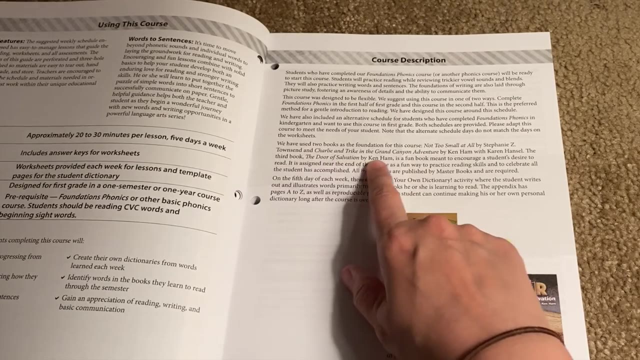 um homeschool mom problems, right, okay, so um, it says we have two books as the foundations of the course- not too small at all- and charlie and track in the grand canyon adventure um. the third book, the door of salvation, is a? um book meant to encourage a student's desire to read. it's assigned near the end of the course. 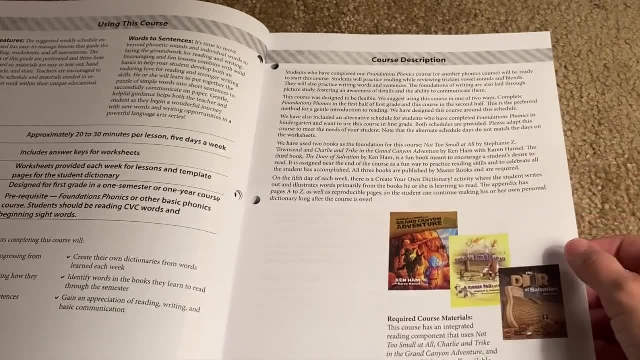 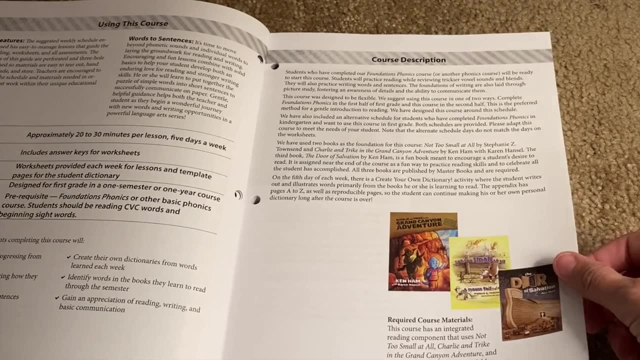 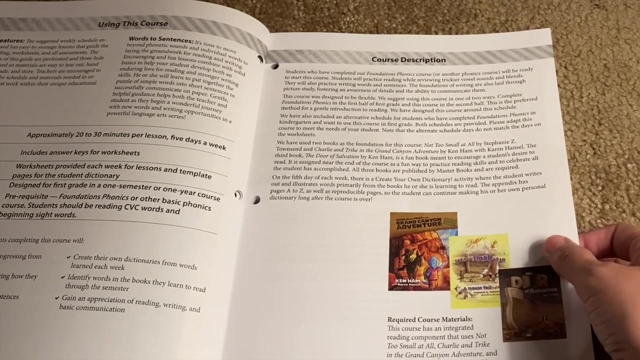 is a fun way to practice reading skills and to celebrate all the student has accomplished. all three books are published by masterbooks and are required on the fifth day of each week. there is a create your own dictionary activity, where the student writes out and illustrates words primarily from the book he or she is learning to read. the appendix has pages a to z as well. 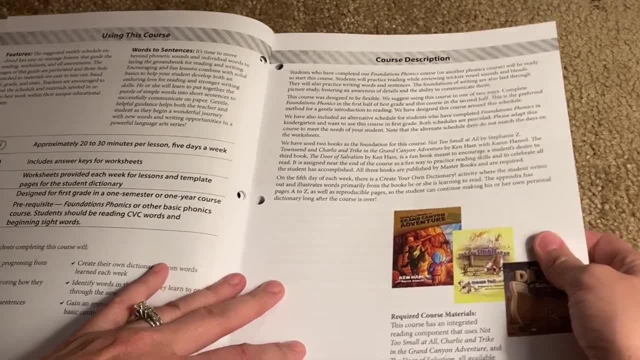 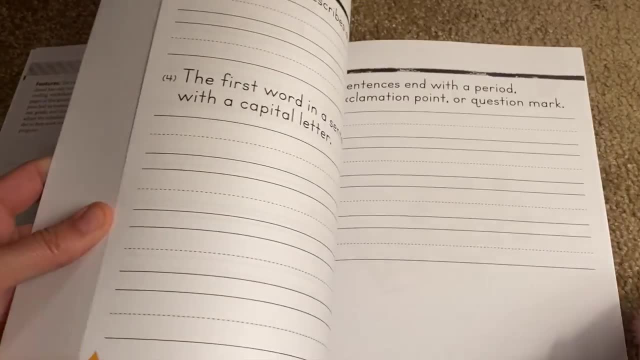 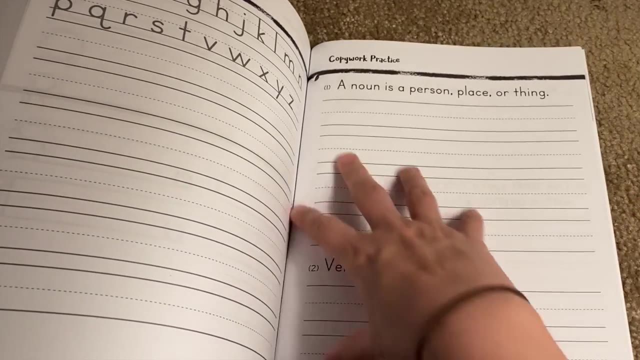 as reproducible pages so the students can continue to make his or her own special or own personal dictionary long after the course is over. so since i am reading that, so obviously the answers to everything are back here. um, but since i was just reading that, i'm going to show you kind of the appendix area. um, so these are copywork pages. 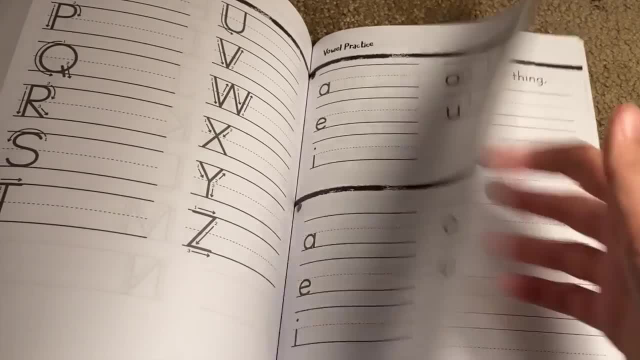 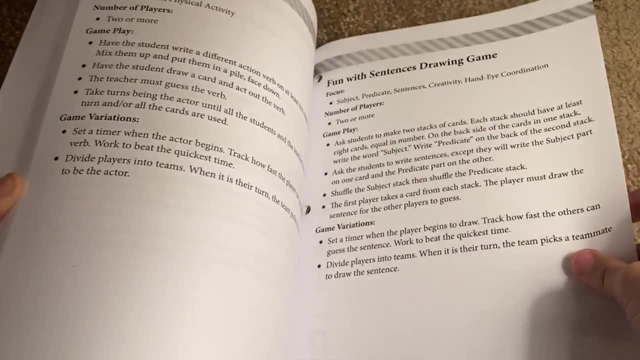 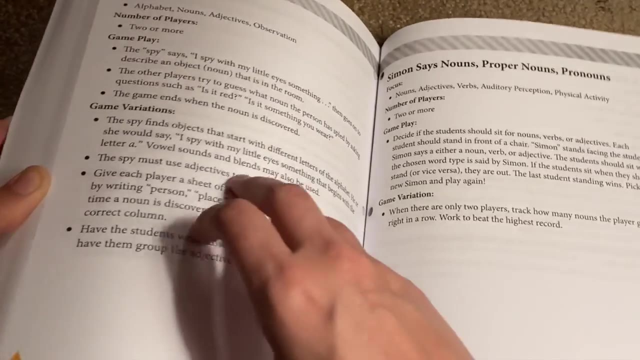 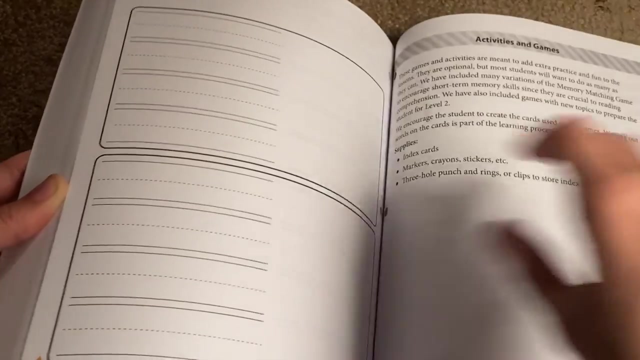 here consonant and vowel practice sheets, extra alphabet writing practice, um fun sentence drawing games, action verb charades. so this looks like just extra activities that you could do. nouns, proper nouns, pronouns. so, as you can see, this is also telling you kind of what they will be learning. so activities: 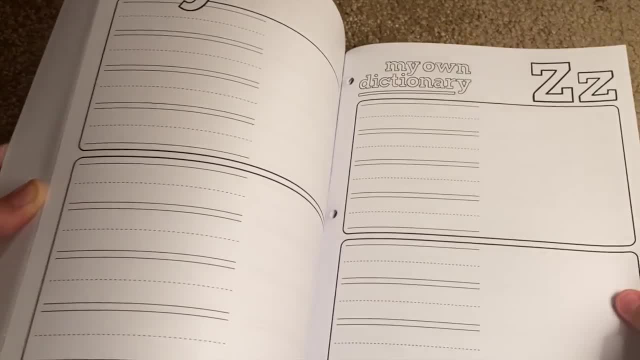 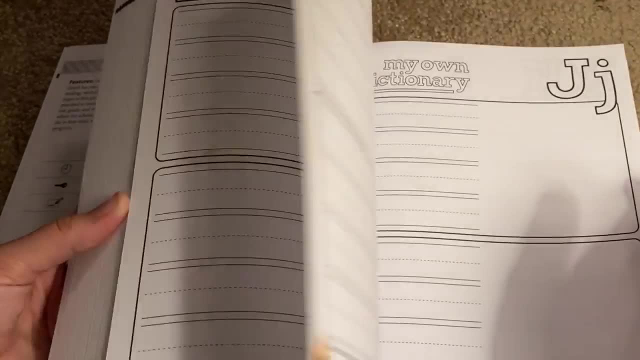 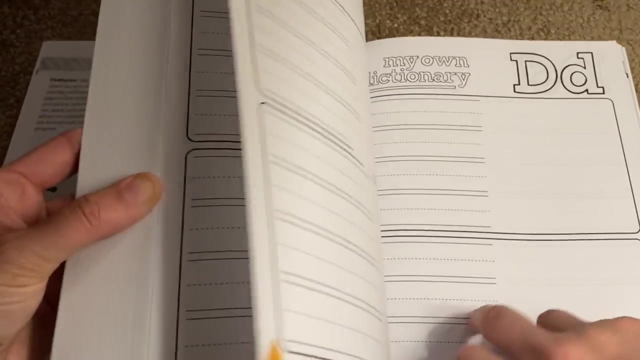 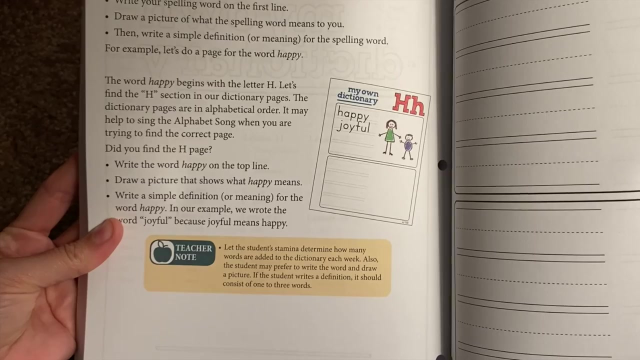 and games. yeah, okay, so this is the my own dictionary pages that they will be filling out each time, and they are all in the back of the book. this is a pretty big section of the book, actually. let me show you how much that takes up, so, um, and it gives you all the directions for creating your own dictionary pages. 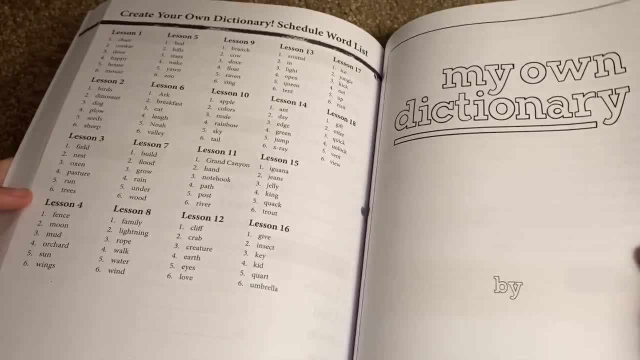 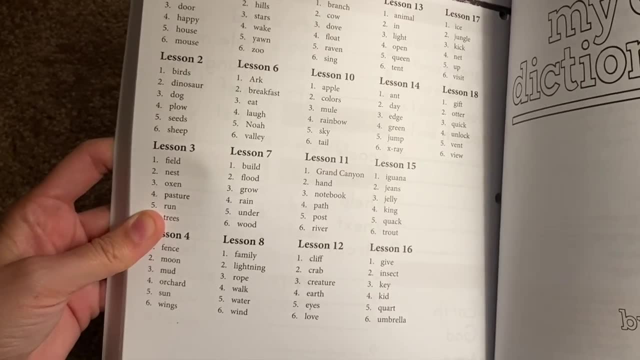 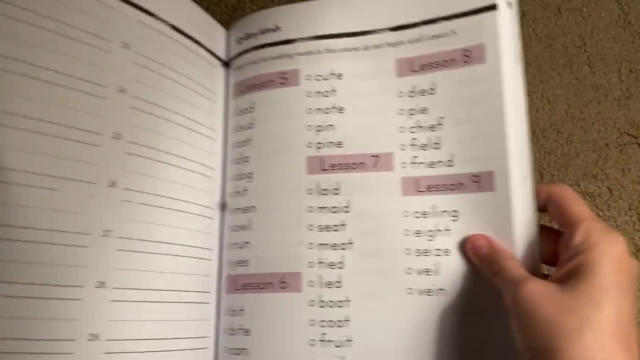 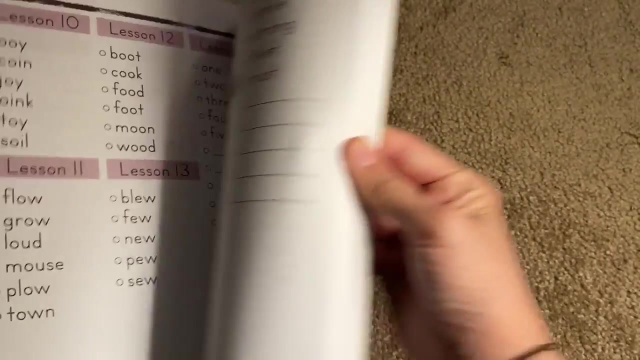 and um. these are the create your own dictionary schedule, word list and um. so you have that there as well. and then these are the spelling words broken down and you can read them if you want to, broken down by lesson, So it looks like they don't start until lesson five And it gives you 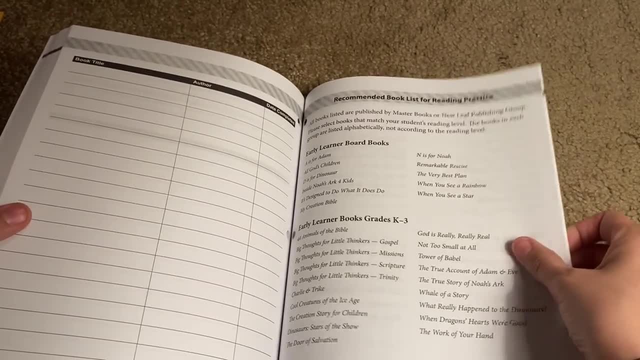 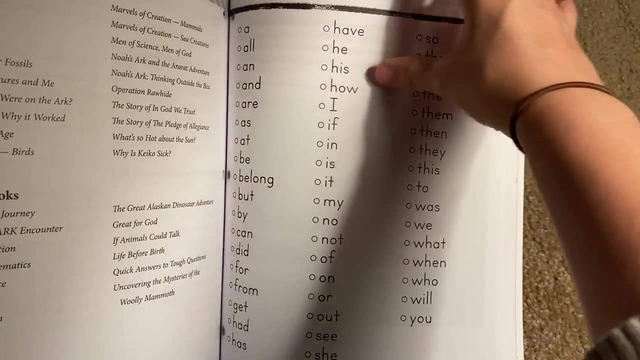 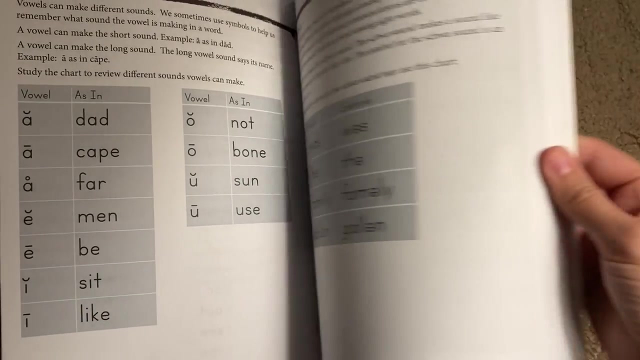 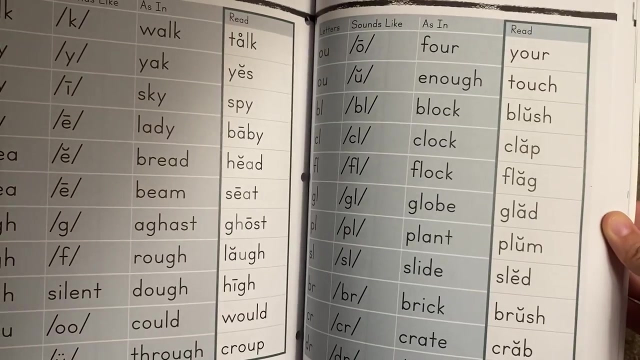 directions on when to do each of these things. So these are just some recommended books for reading practice. if you want some other recommendations, Sight words that they will be using and learning Phonics review pages, Phonics charts- So everything is just laid out really well. It's very easy to read. 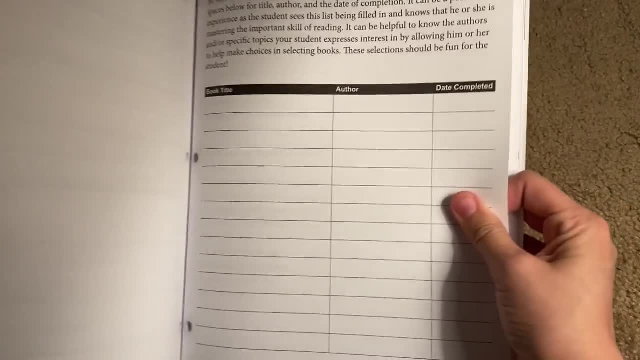 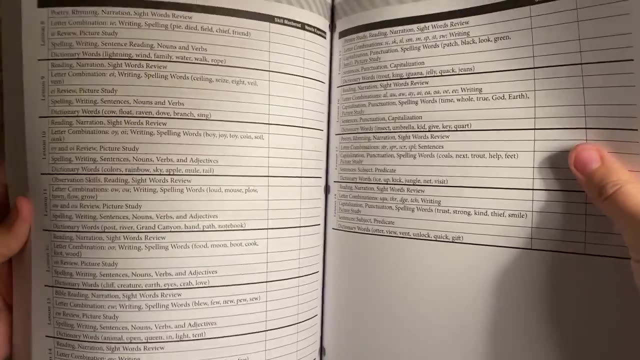 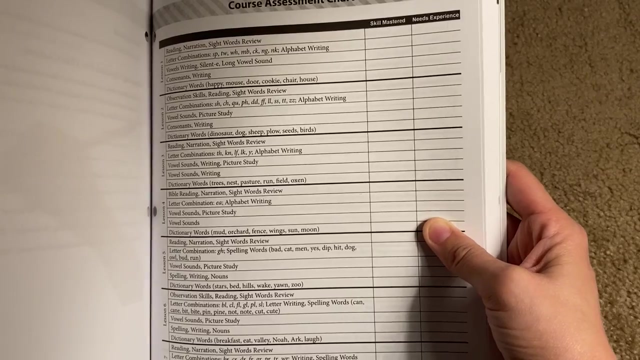 Okay, and then this is just a little reading book or a book reading list that they can keep record of. Okay, so here we have assessment charts as well, But let's go back to the beginning so I can show you, And this gives: 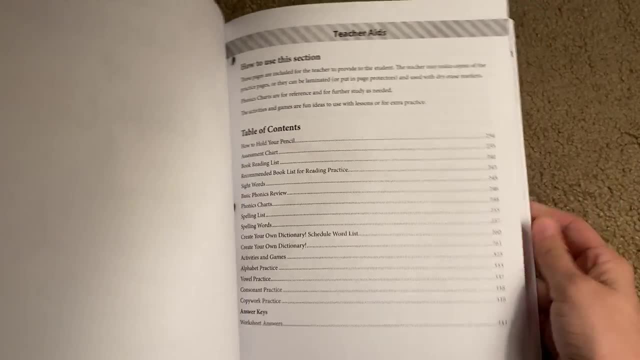 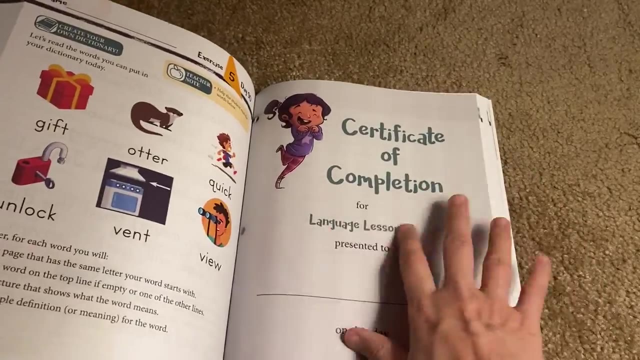 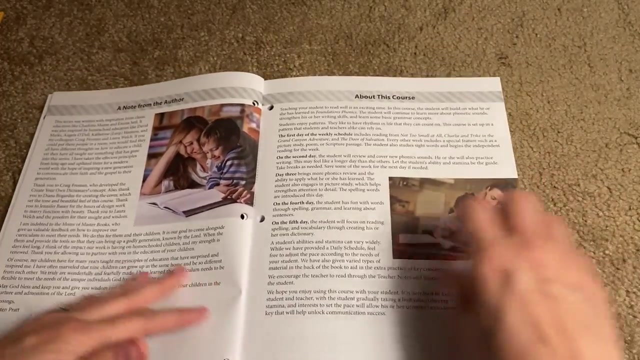 more examples of assessments and tells you how to use this whole section. I probably should have started right there. So all right, And they even get a little certificate when they're done. Okay, so let's go back to the beginning here. So on the first day, 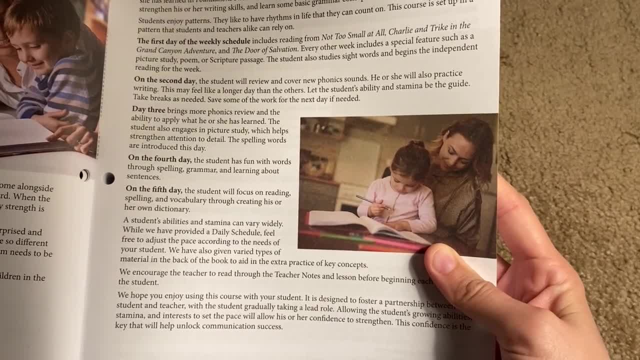 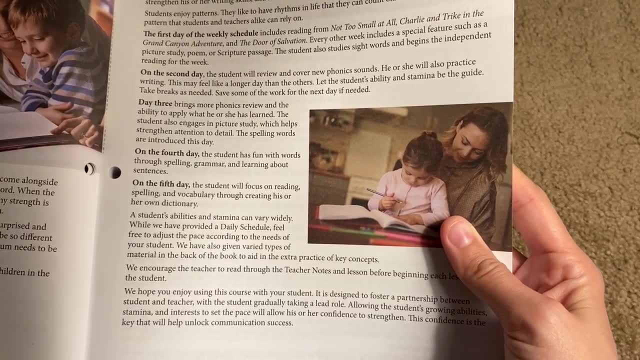 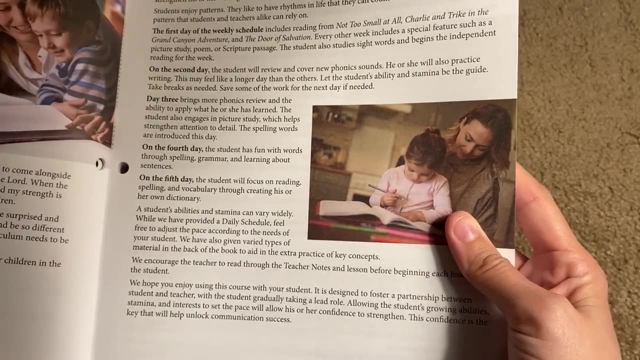 you read from, Not Too Small at All: The Grand Canyon Adventure and The Door of Salvation. Every other week includes a special feature such as a picture study, a poem or a scripture passage. The student also studies sight words and begins the independent reading for the week. 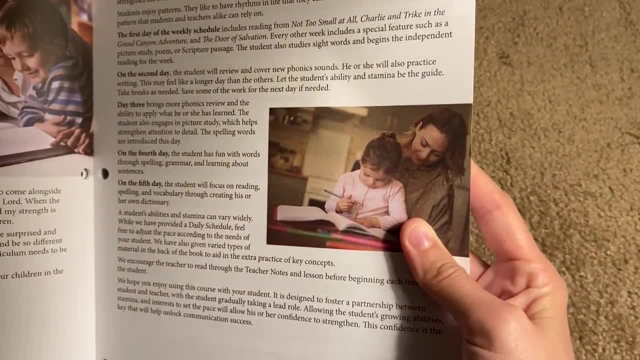 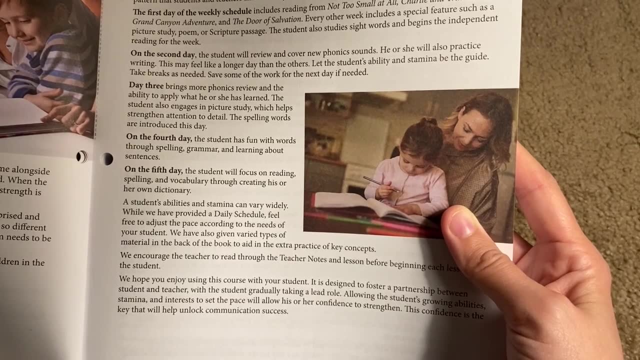 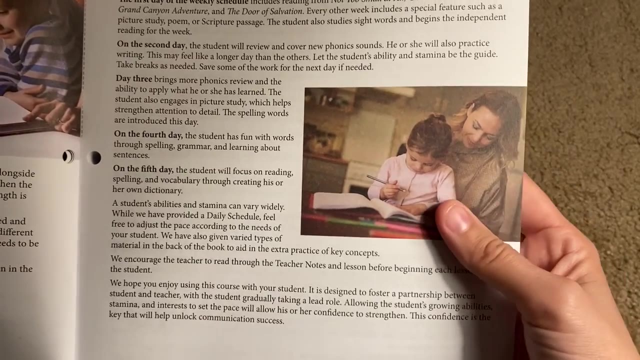 So they do not read the whole book every time. I'll show you how they break it down. On the second day the student will review and cover new phonics sounds, practice writing. it says the second day may feel longer. Let the student's ability and stamina be the guide. 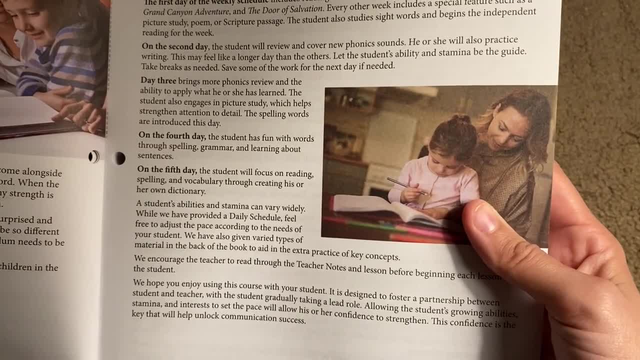 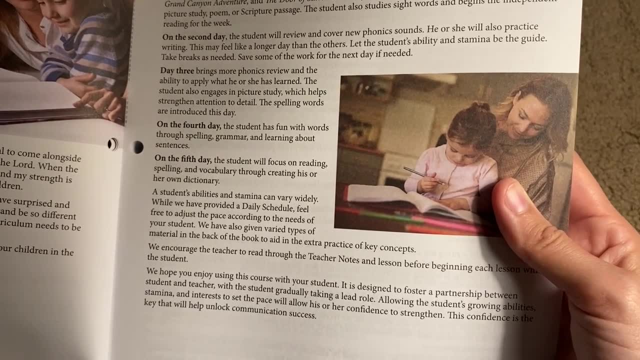 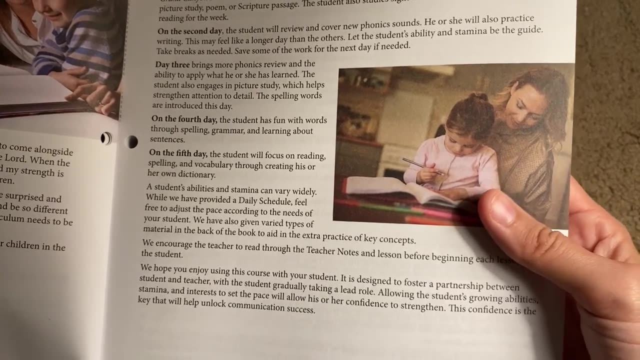 take breaks as needed. save some of the work for the next day if needed. Day three brings more phonics review and the ability to apply what they have learned. The student also engages in picture study, which helps strengthen attention to detail. The spelling words are introduced on: 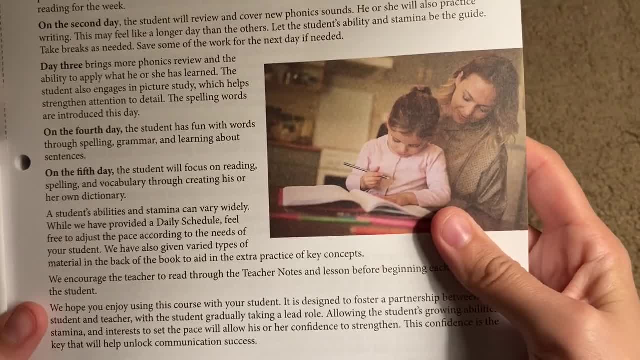 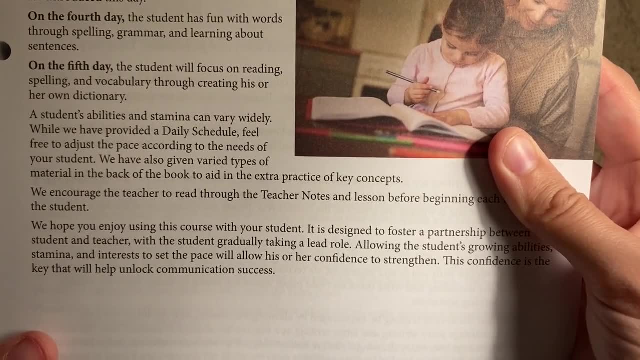 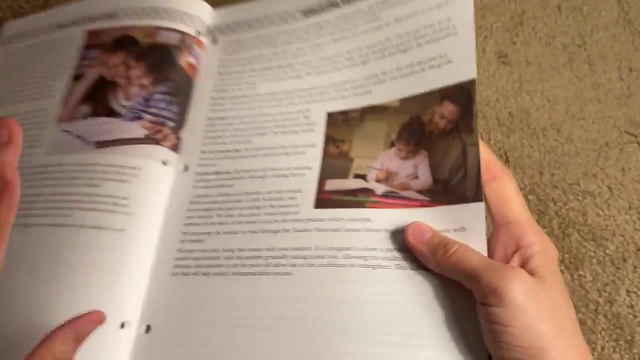 the third day. On the fifth day, the student has with words through spelling and grammar, and learning about sentences. On the fifth day, the student will focus on reading, spelling and vocabulary through creating his or her own dictionary. So yeah, so that's kind of a breakdown of how the days work, So it's very informative for 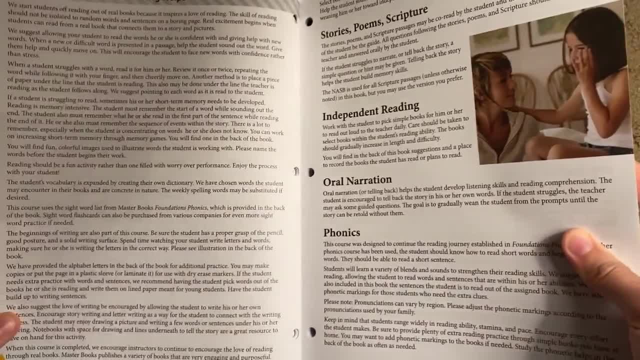 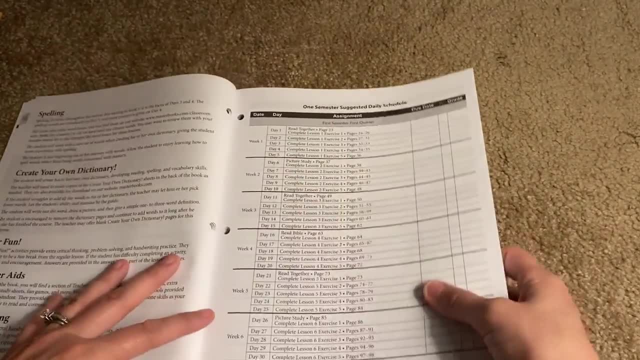 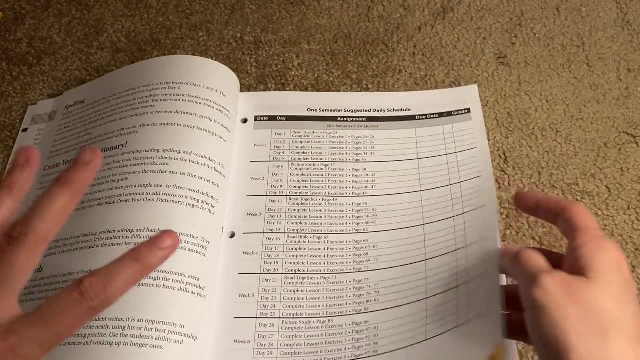 everything. So if, especially if you are new to teaching or homeschooling or anything, this is a super user-friendly curriculum. This is like literally an open and go curriculum. I used to teach public school, but I have learned to really appreciate this as a very busy mom of so many kids. 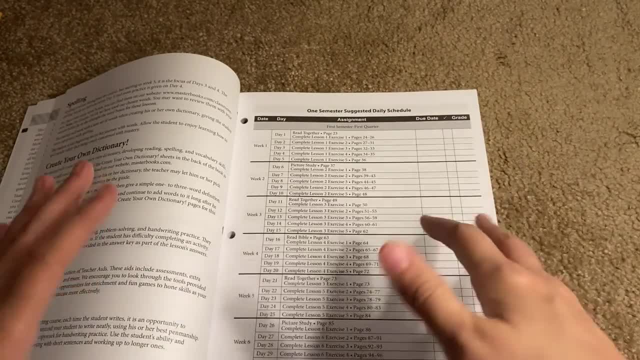 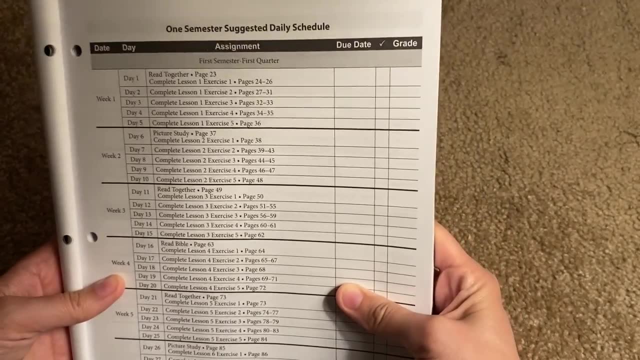 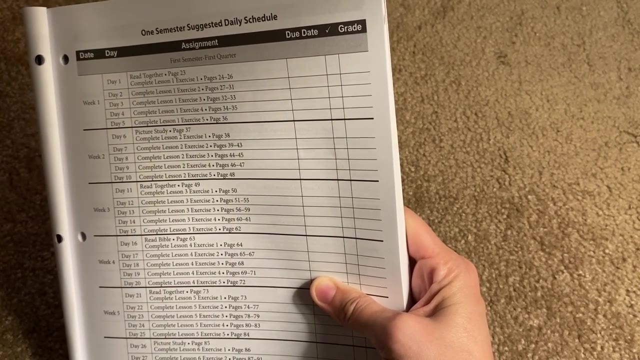 especially since I'm homeschooling multiple kids, I'm really starting to adore and love this curriculum. So okay, so here we have. I really like this, because I am not a by the book kind of person Actually with with homeschooling. 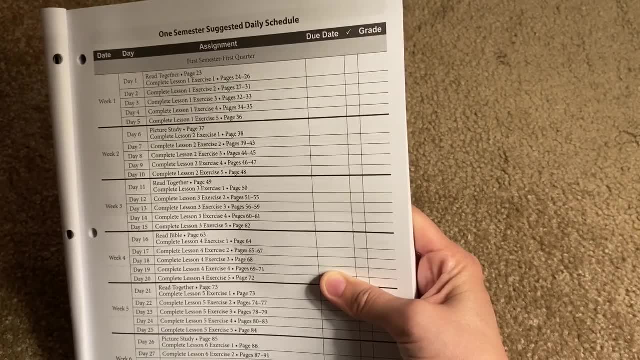 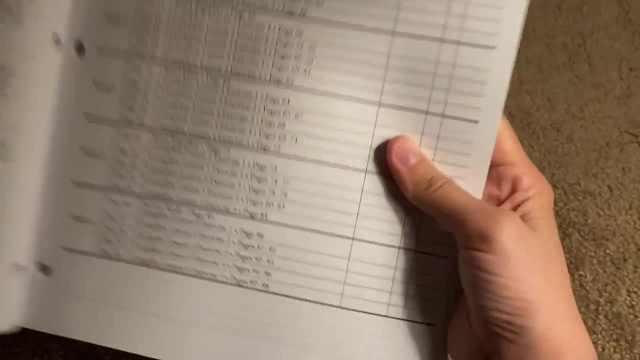 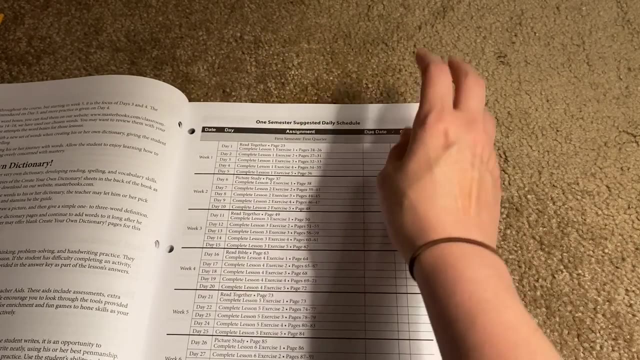 I am pretty Charlotte Mason minded. However, there are some times that it feels good just to put a check in the box, And so that's one of the things that I like about this is how it's laid out so well and so simple, And you can literally just put a check beside it. Now, I don't use the due. 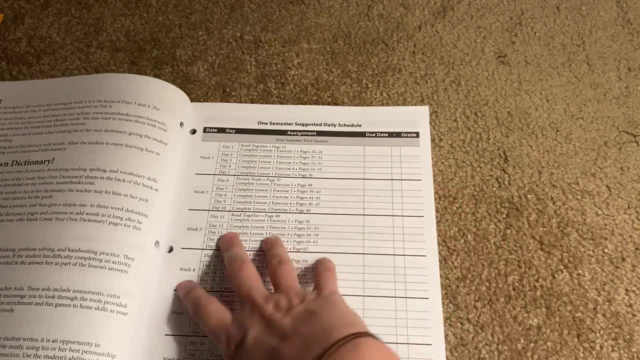 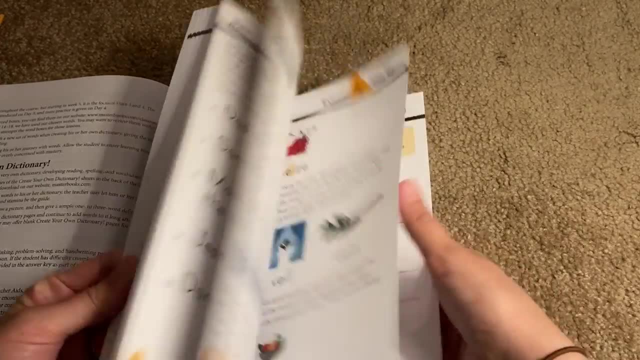 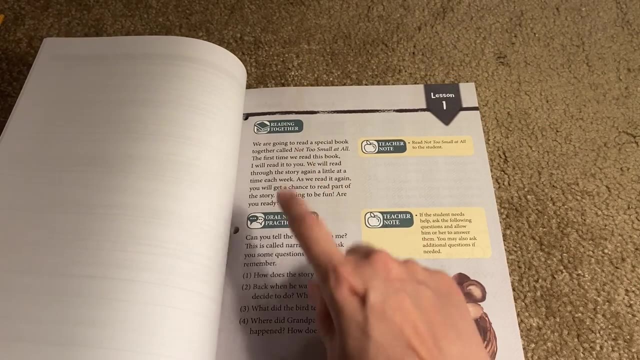 date lines, and I don't normally put the grade there, But that option is there if you want it. So you read together page 23.. So I'll kind of show you how you would do this, So you would read this together. Then they do a little oral narration practice and it has constant teacher. 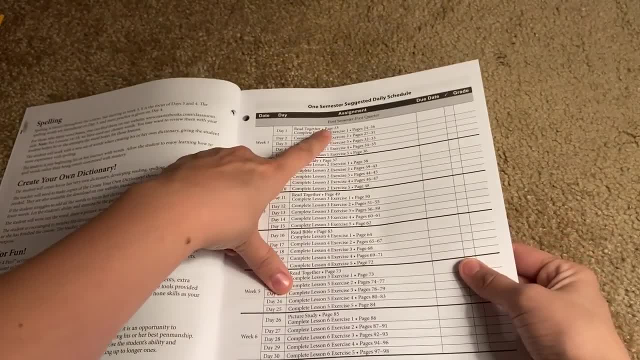 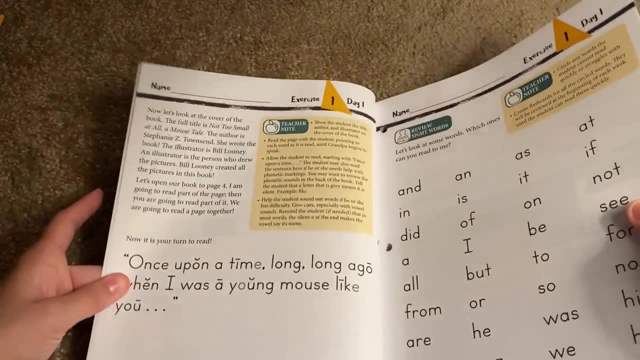 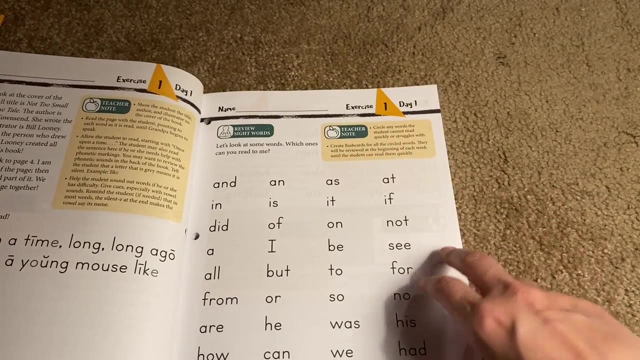 notes. Okay, so you read 23,. complete lesson one, exercise one, pages 24 through 26.. So again, there are teacher notes on there. Okay, so they're looking at the page, And so they're looking at the words. which ones can you? 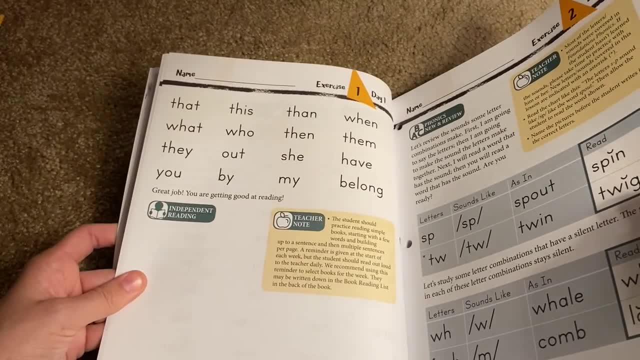 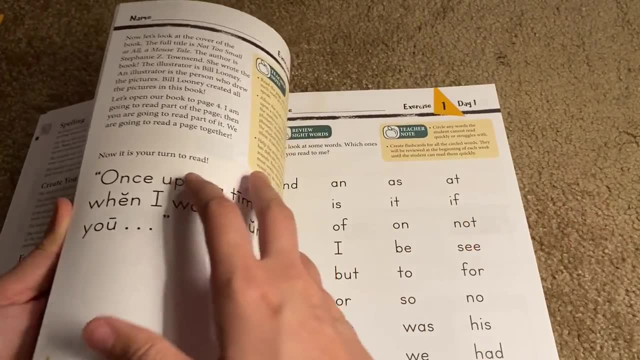 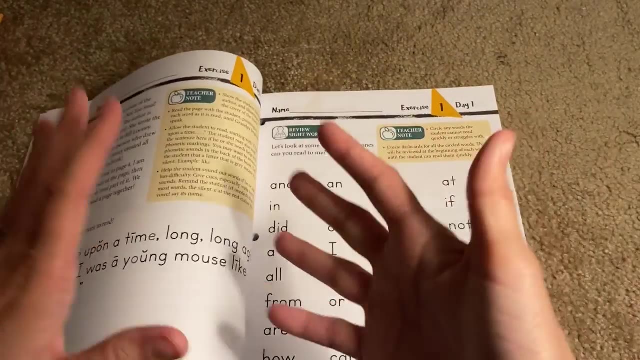 read to me: Okay, And that's the end of day one, Okay, So obviously they're not just going to complete those pages that it's having you. it's prompting you to do different things, And, and what I like about this curriculum is that it lends itself to always be expounded upon. 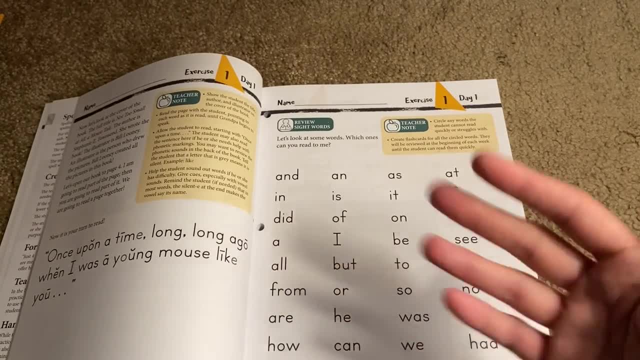 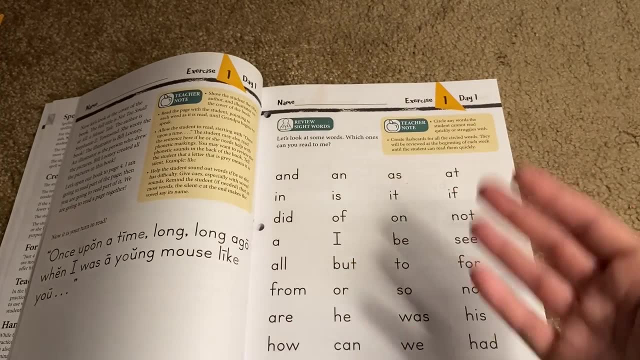 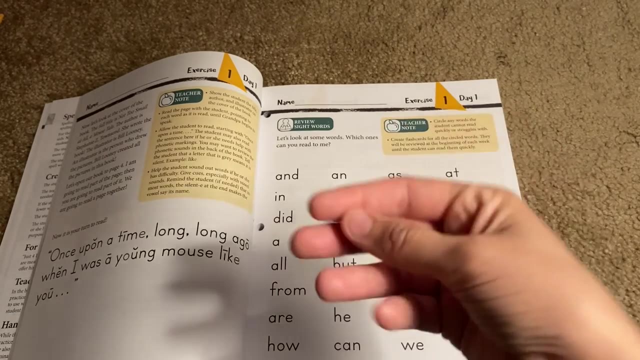 So it's very easy to add fun little activities to without having to draw out your day really really long in this subject. So you get down to the nitty gritty here with this and then it gives you the time and availability to do all the fun learning activities to reinforce this kind of. 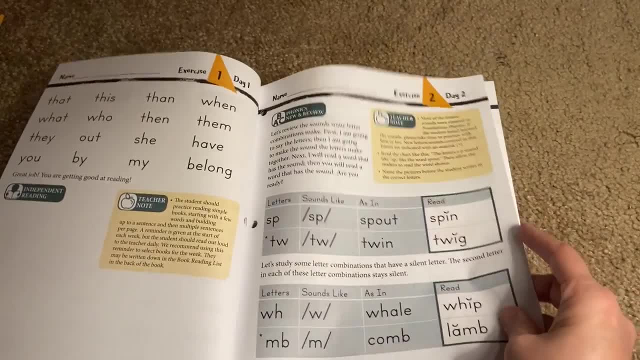 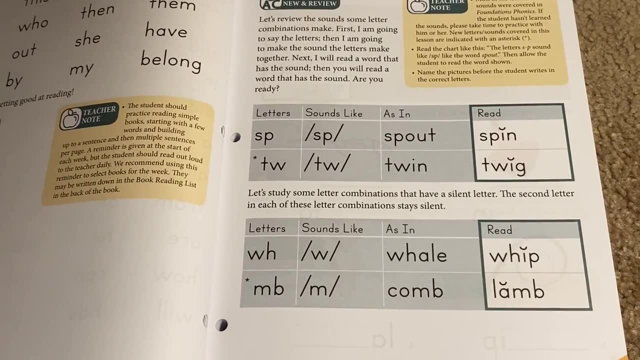 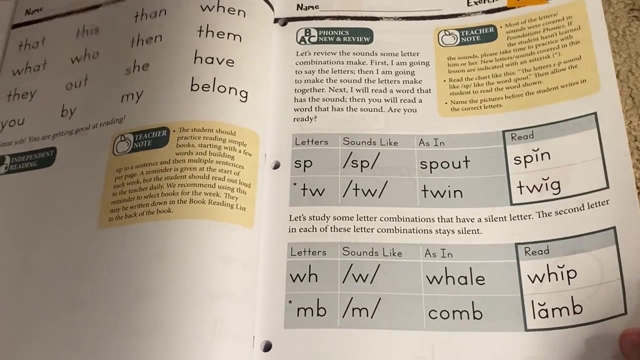 stuff. So that's one of the reasons that I like this. So I'm just going to flip through here And let you guys see. let's see if I can get this a good picture in the frame here. Let you guys see, I'm just going to kind of flip through and kind of show you what some of this looks like. 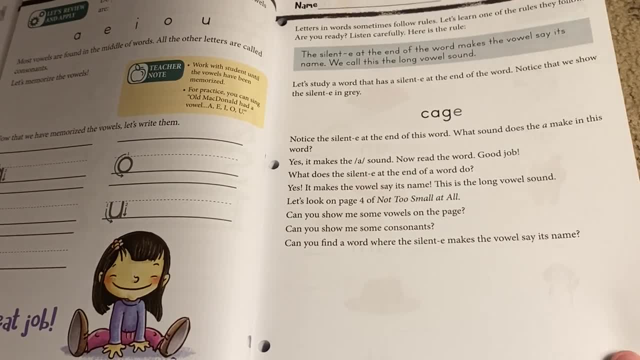 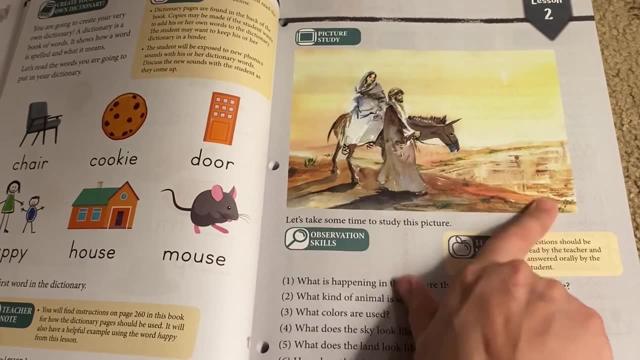 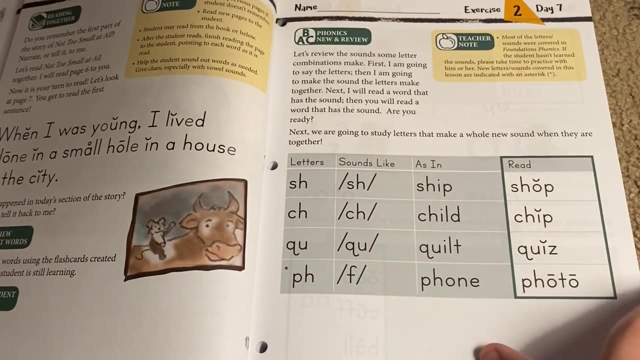 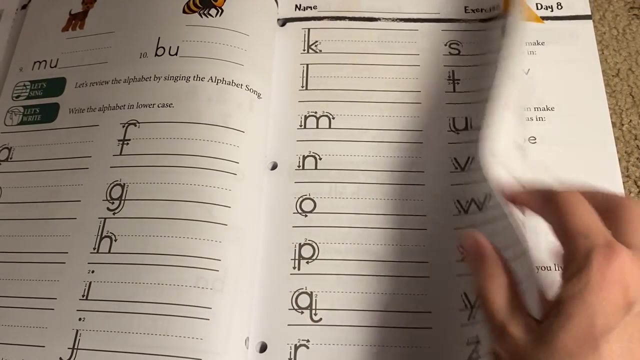 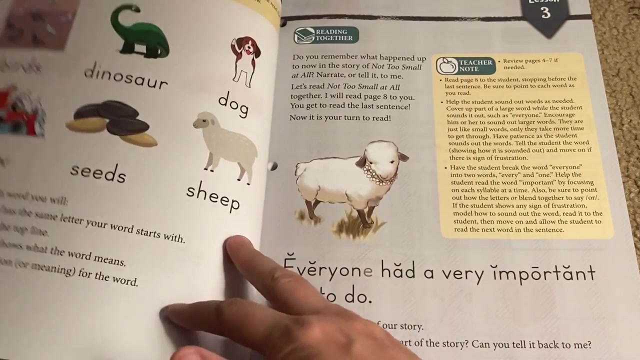 And all the different things that you're going to be doing with them. So looking for missing letters. there are picture studies within this, which I think is really cool. Let's see Handwriting practice. I just like how simple it is. It's just laid out really well, But it's just so thorough And I know. 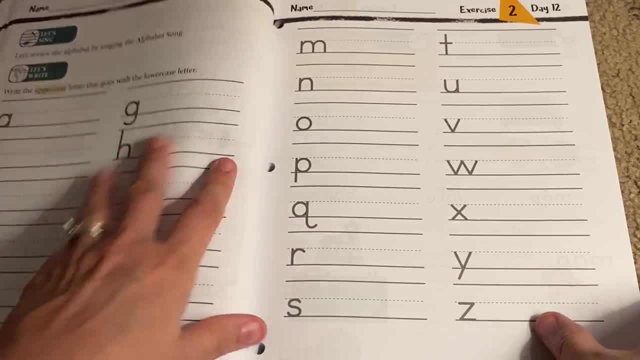 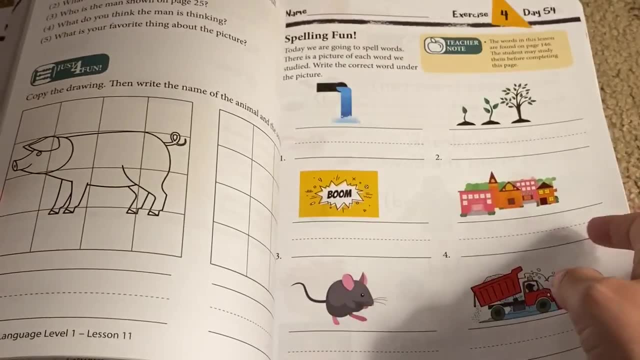 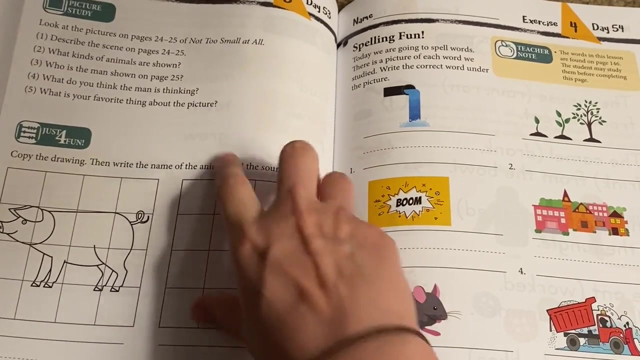 I keep saying that, but that's just really how I feel. Um, so let's turn now to kind of like: midway through, there is again a picture study in the- in a book this time. So there's a picture study in a book. 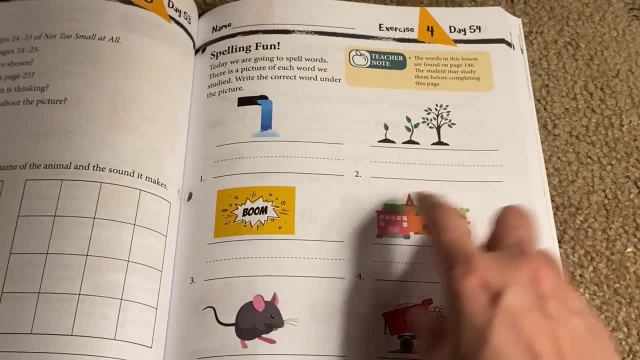 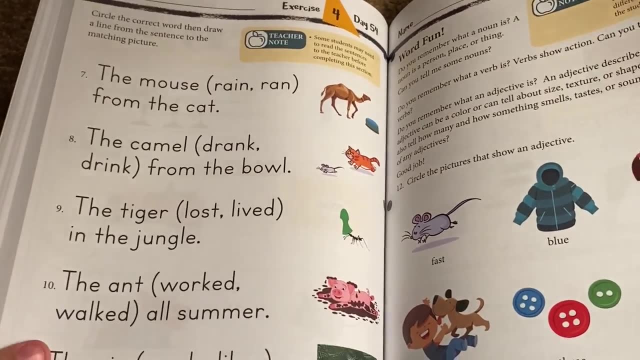 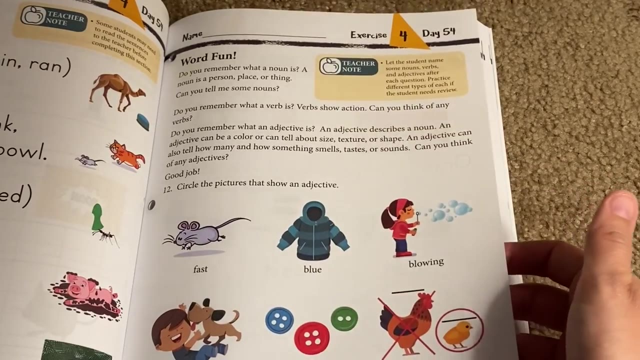 and then it has them copying and drawing um fun spelling circle, the correct word. then draw a line um from the sentence to the matching picture: Wordfun, fnt, fnt, so talking about nouns. so it does some grammar in there. 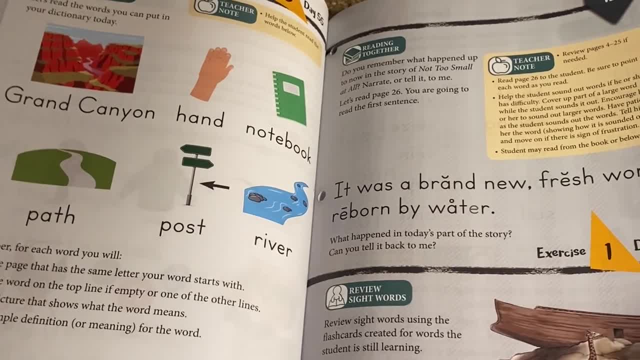 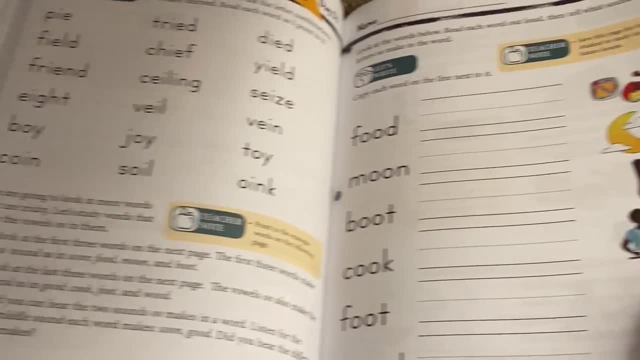 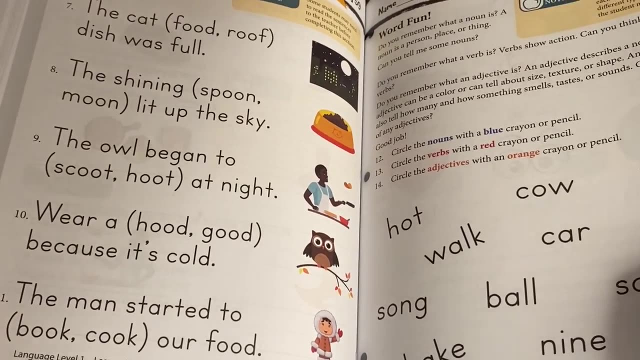 and so let's read the words. you can put them in your dictionary. today i'm just super excited about this. i think it's going to be great. i can't wait to see colleen's video, to see it in action. she's going to show what that lesson looks like with sophie. 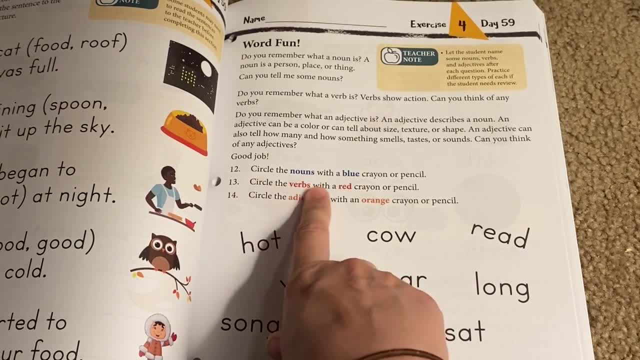 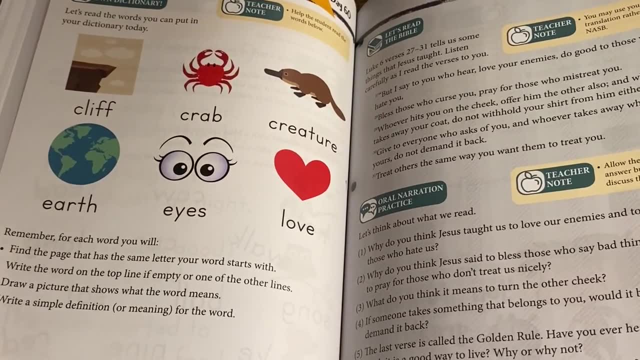 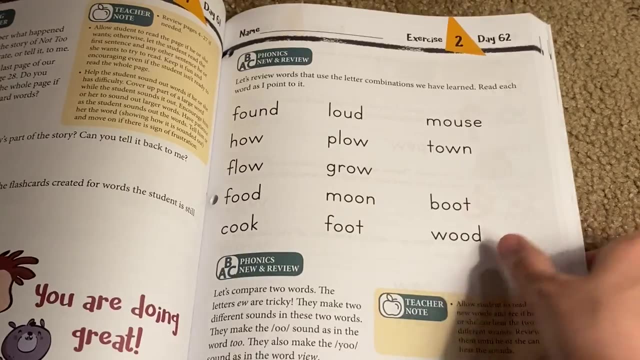 so circle the nouns with blue crayon, circle the verbs with the red crayon, circle adjectives with orange. so it's getting them, seems like it gets them pretty well acquainted. but what i also love about this is that it is so biblically focused. that is one thing that we are loving about. 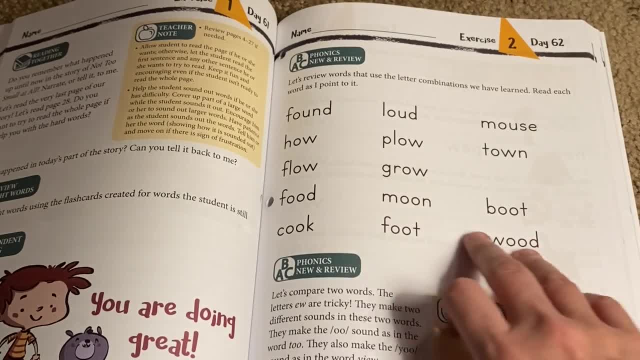 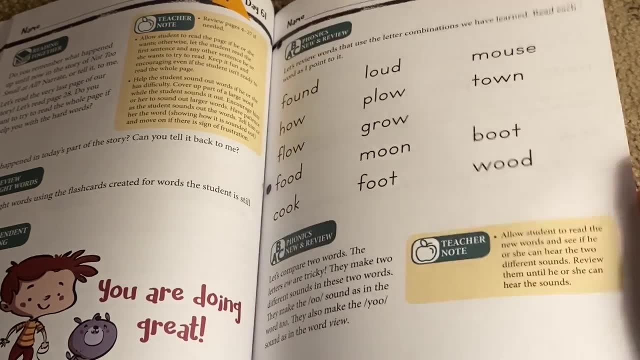 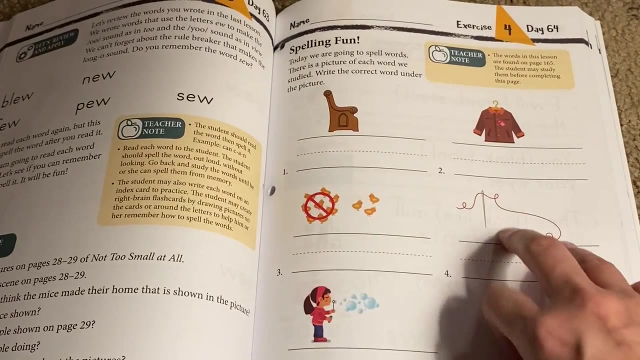 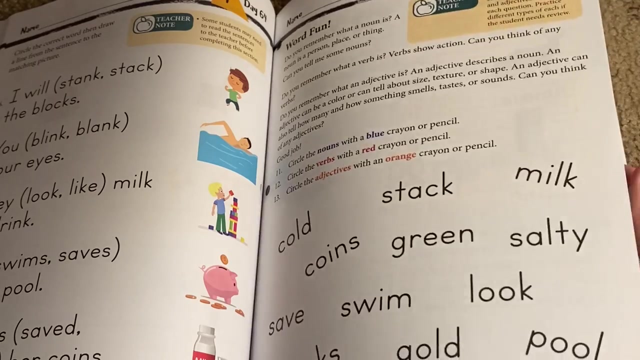 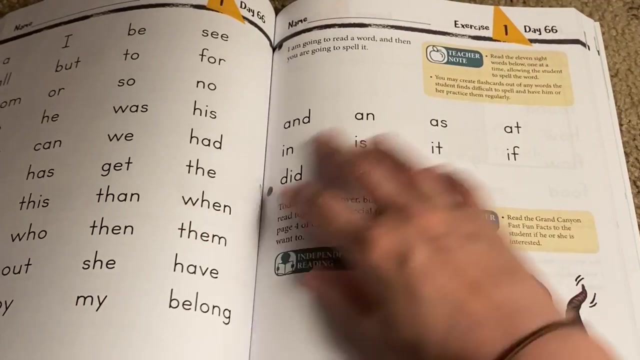 foundations. phonics is just how biblically focused it is and i just i love that. it makes it such a sweet time um with me and my kids engaging and and talking about um scripture. so okay, and again with the nouns, verbs and adjectives, and then 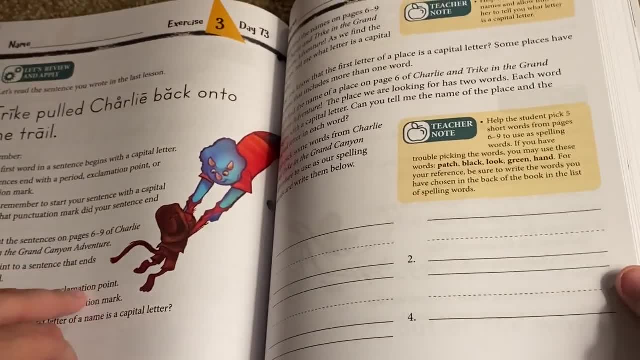 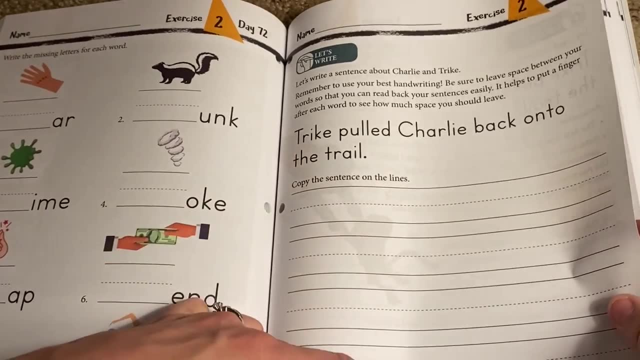 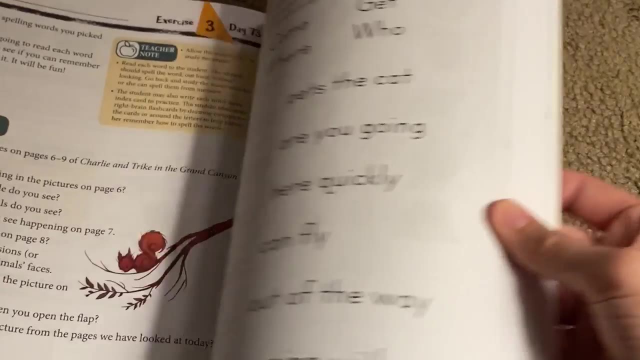 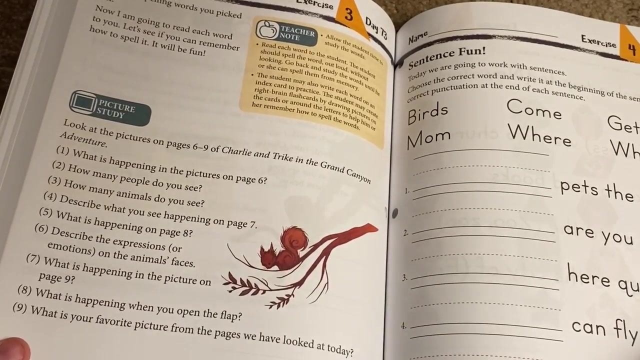 okay, so let's go again. hold on track, pulled charlie, okay. so here they're copying the sentence. let's see completing the sentences. look at the picture in charlie and track what's happening in the picture. how many people do you see? how many animals? so, and then some comprehension. 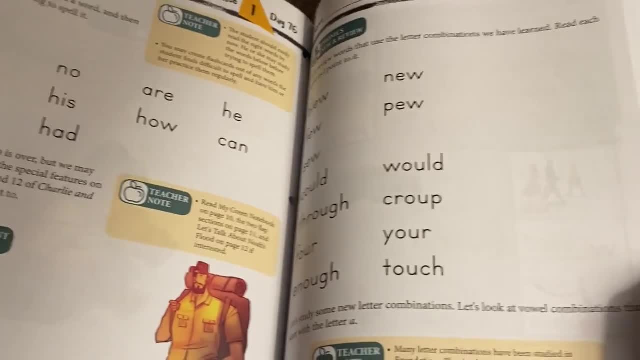 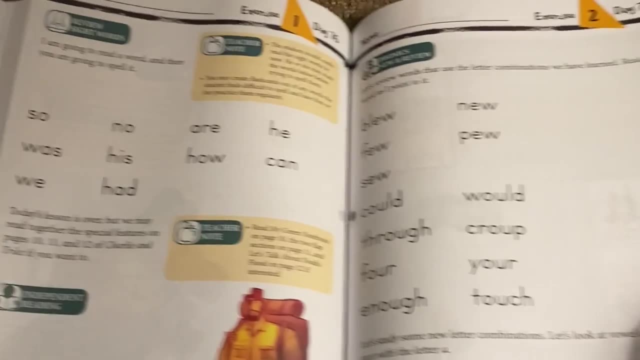 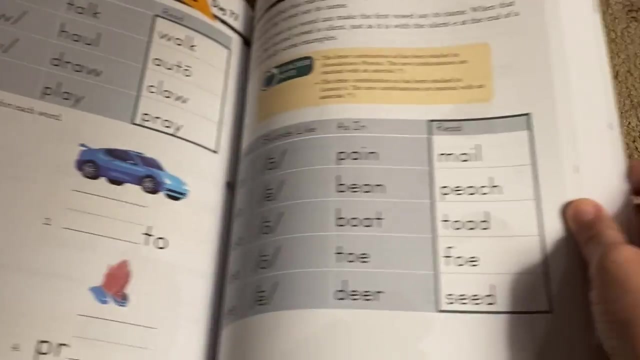 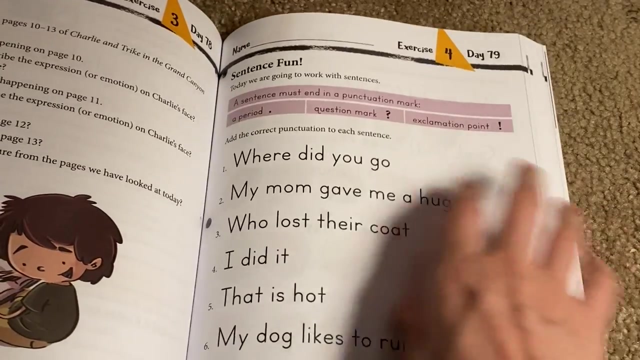 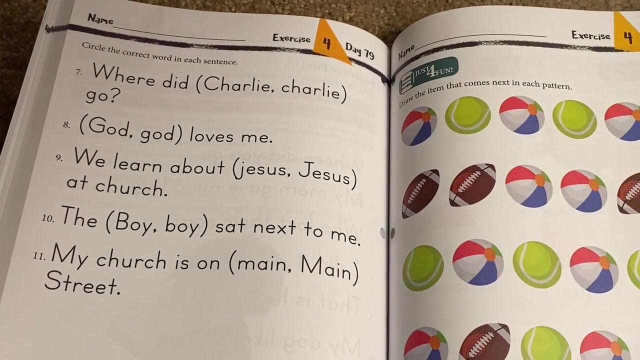 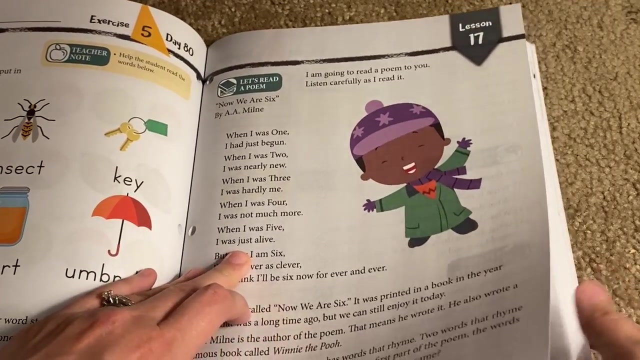 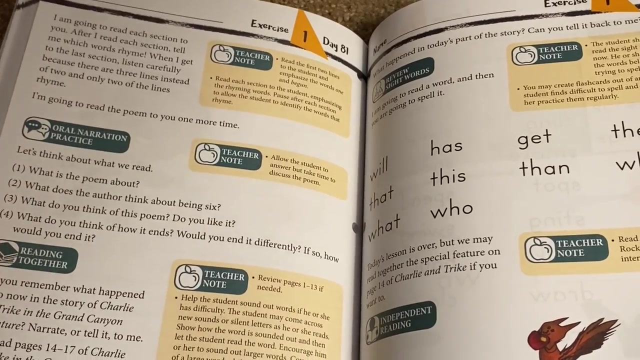 stuff: Phonics and New Phonics, New and Review, Review, SotWords, Independent Reading And then some more. so here we're talking about punctuation marks and then looking at capitalization and patterns, and then reading poems And some more narration reading together. 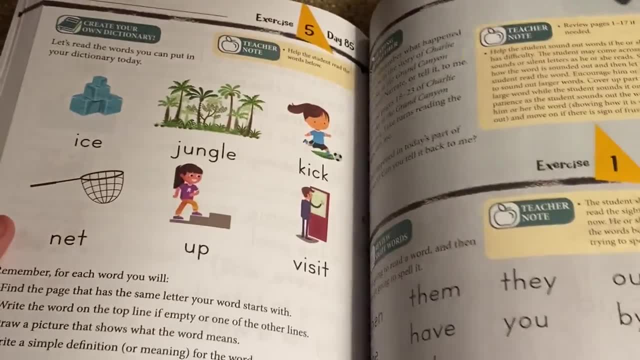 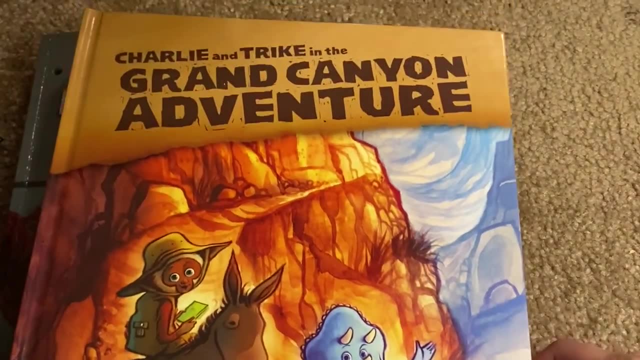 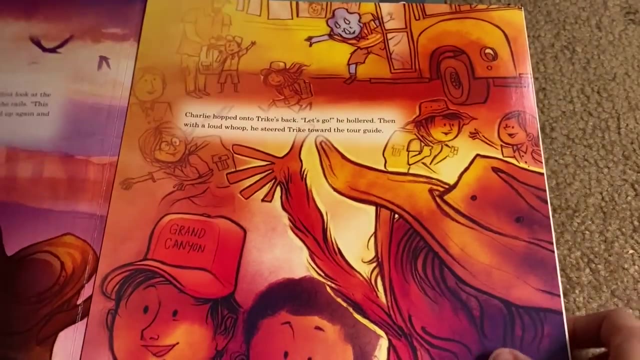 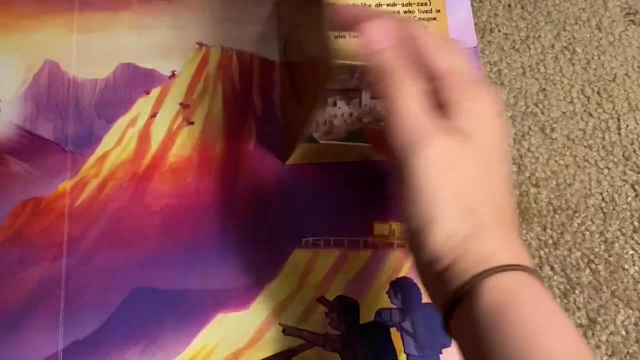 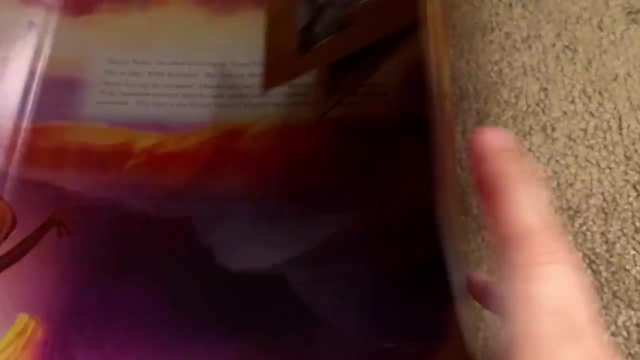 So I think this will be just wonderful. I cannot wait to start this. So this is Charlie and Track in the Grand Canyon Adventure. So these books just look really cool. So this opens up and then they can look at pictures and fun facts about the Grand Canyon. 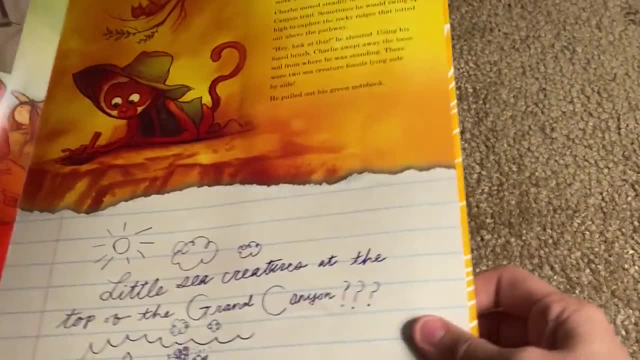 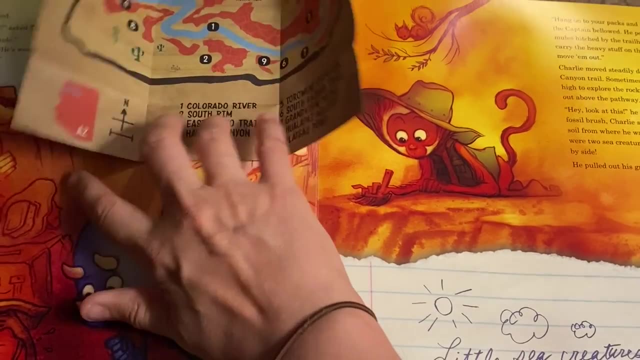 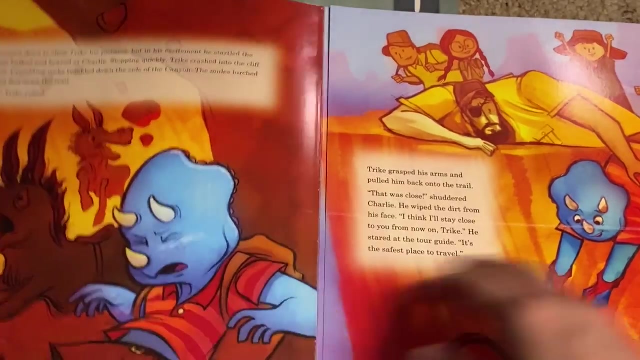 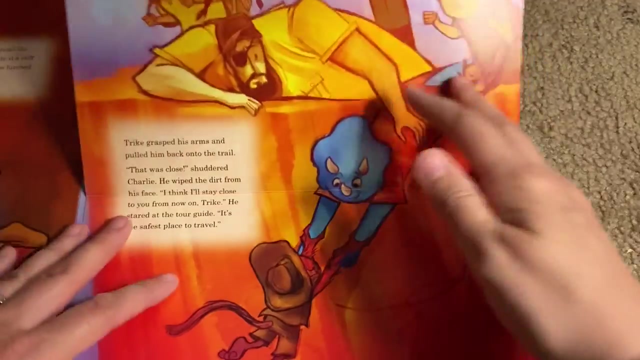 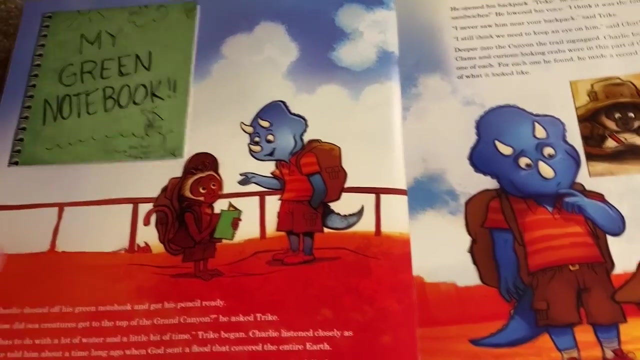 Oops, make sure I close that- And then a Grand Canyon map, which I thought that was really cool. So it's kind of some little interactive books here. Okay so, and there's more, I'm just not going to go through the whole thing. 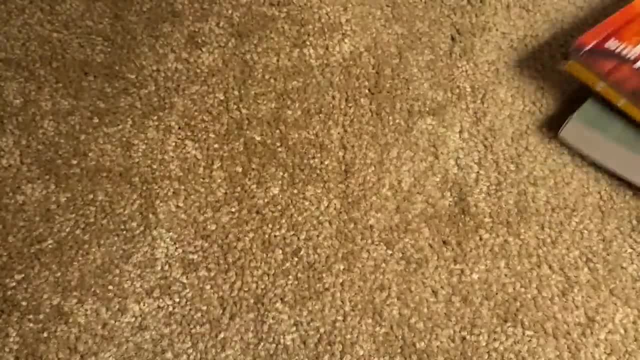 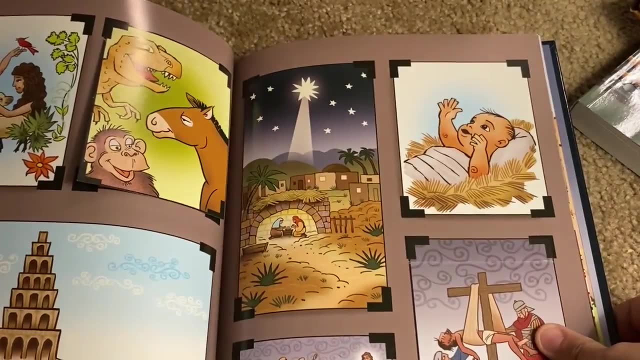 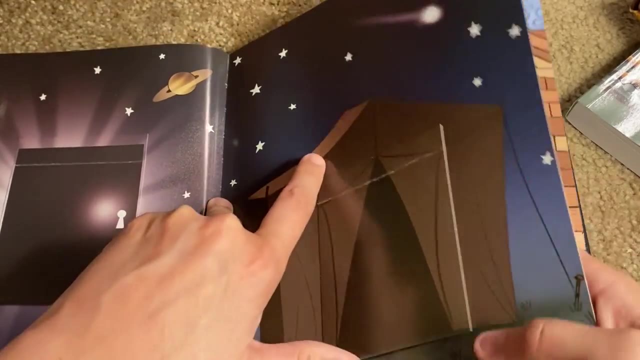 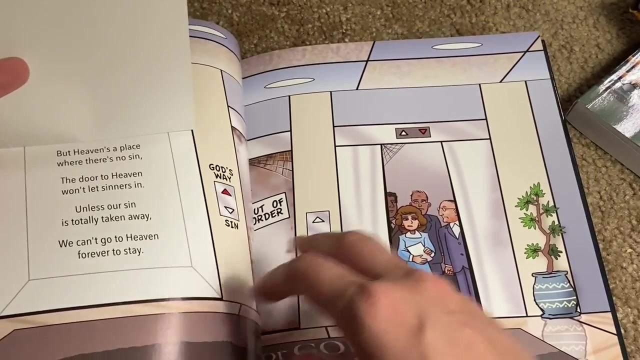 So that's one of the books, that's, that goes along with it. The next one is The Door of Salvation, And this one as well. It's all like little: lift the flap things, All the doors, because it's the door of salvation. 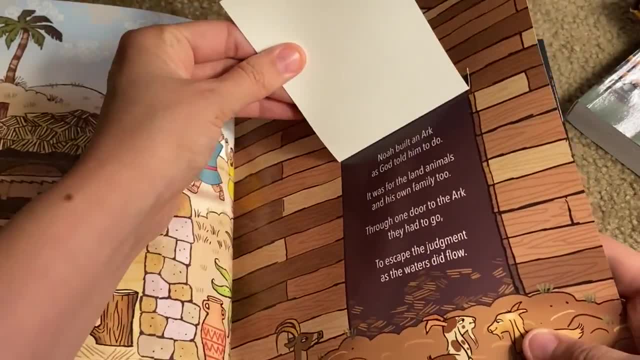 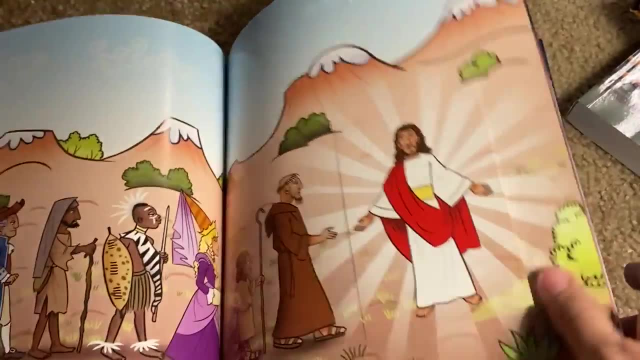 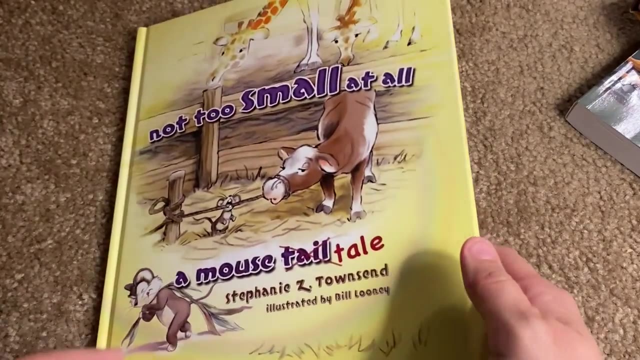 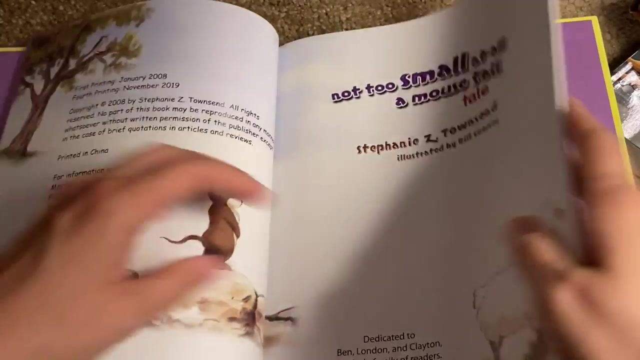 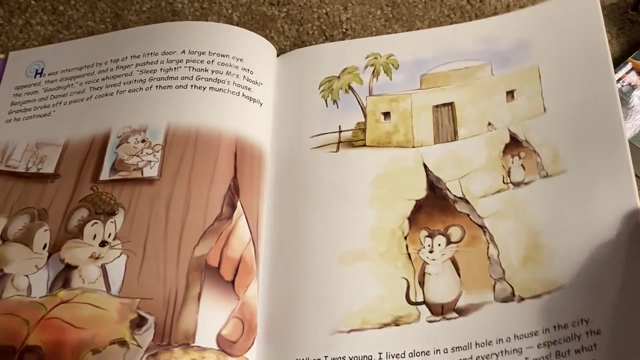 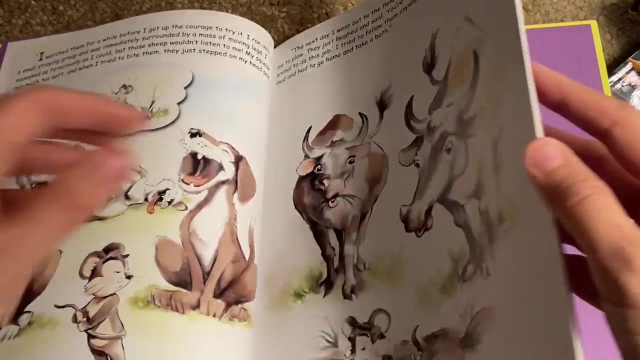 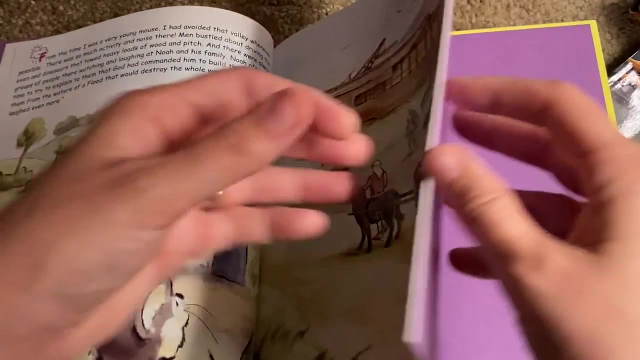 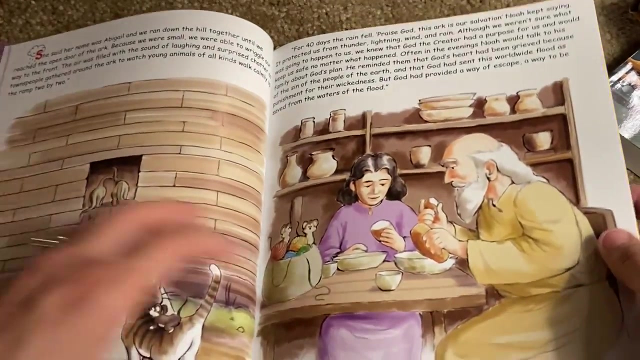 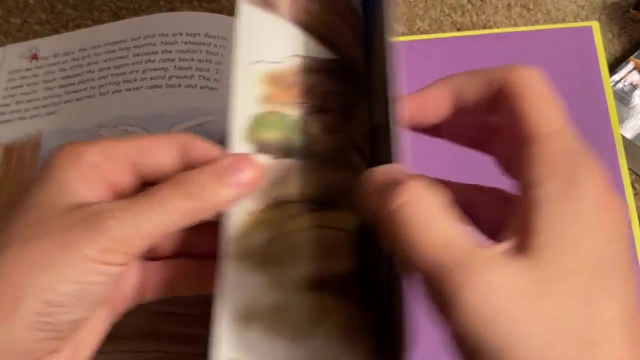 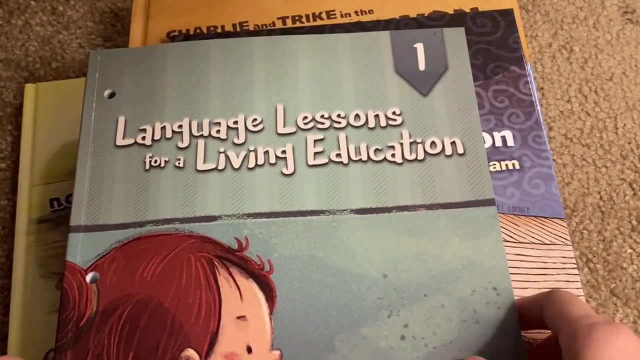 Okay, Okay. So, like I said, there's all these different little doors they open And then, not too small at all, a mouse tail. I like the little illustrations, They're sweet. So obviously it incorporates Noah's Ark. So that is all the components of Language Levels. 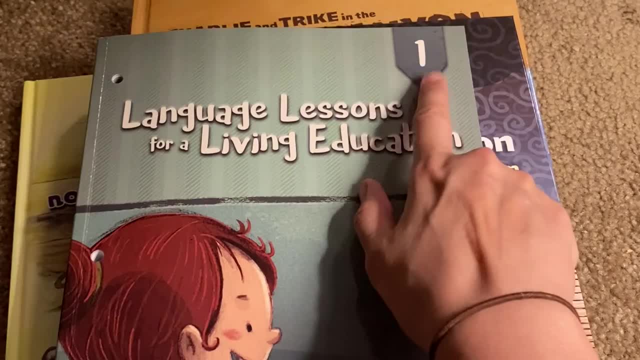 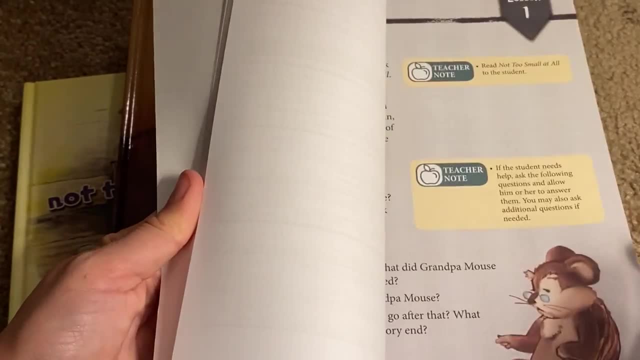 So that is all the components of Language Levels. I'm going to close this video and end it with some time for those of you who wanted to stay with me listening. I hope that this was helpful to you. If there is anything else you have questions about, feel free to put them down in the comments below. 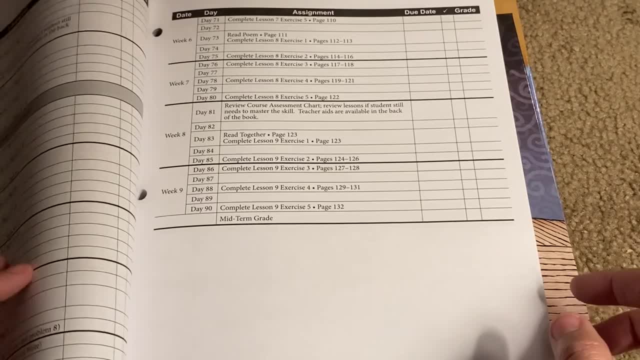 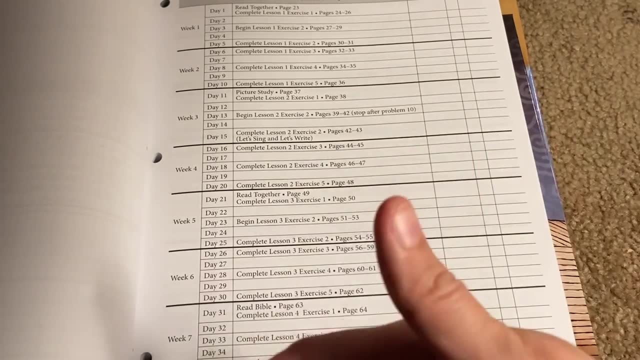 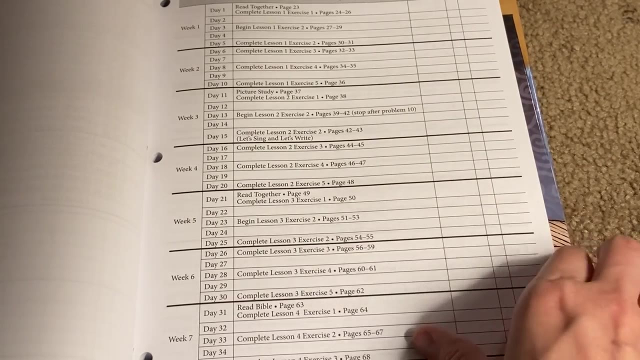 I bought and paid for this curriculum. However, I do have a referral link for Masterbooks. It doesn't cost you any extra to use that referral link, But if you would like to, it does help me out a little bit and then when you, if you order, you will get a referral link.